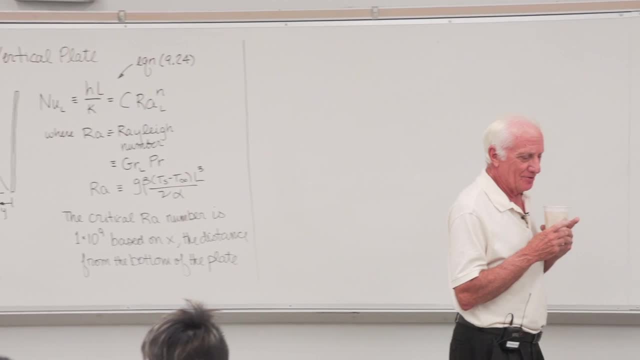 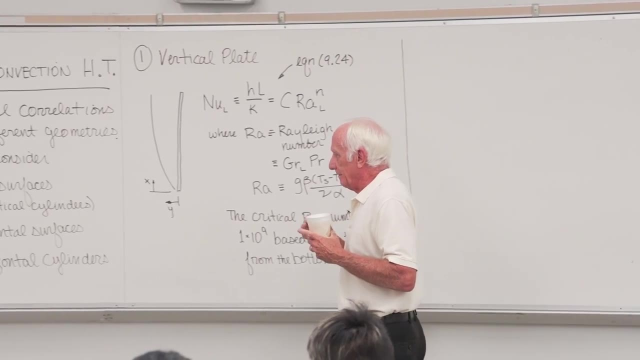 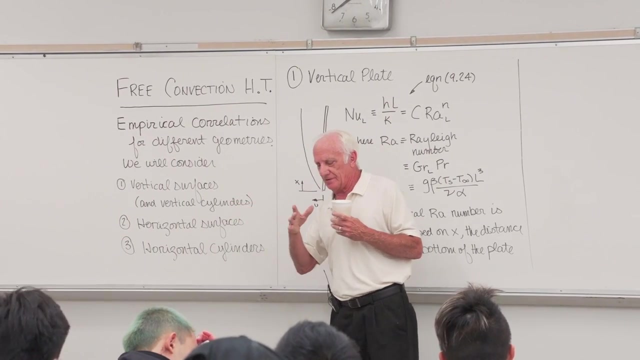 What was chapter seven? Pretty much: external flow over flat plates, external flow over gaussian flow, 1060, 00R, m, m, E, B, O, C over cylinders. what was chapter 8? inside of cylinders and tubes, we're going to consider for free convection three geometries, the they're very popular. 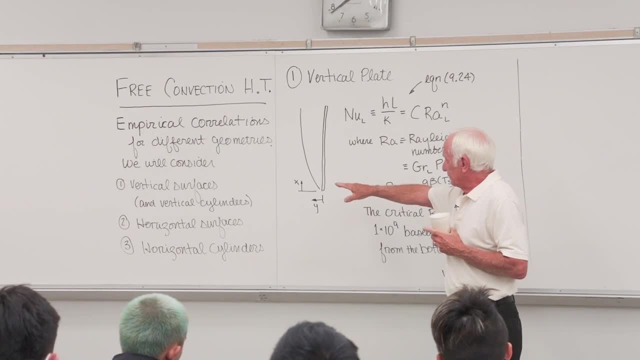 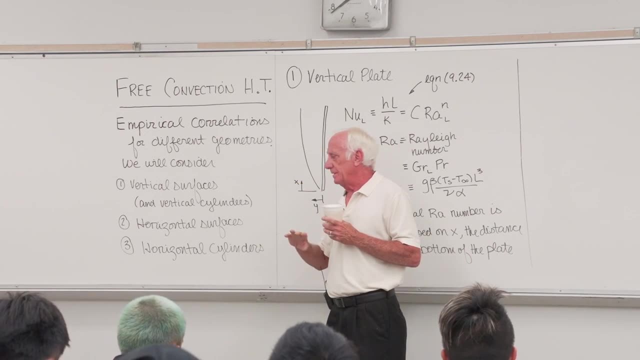 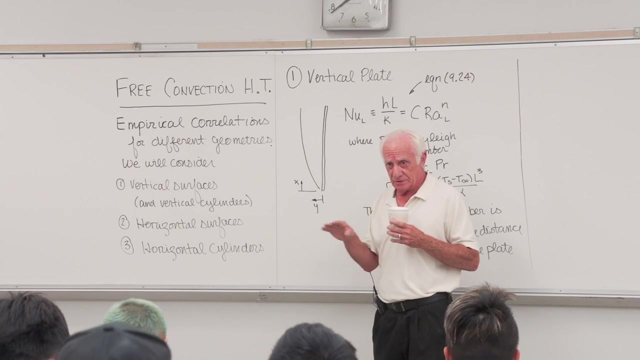 geometries in engineering: a vertical surface, the picture we drew last time. we drew the picture last time, vertical surfaces and maybe, under certain conditions, vertical cylinders. then we'll look at horizontal surfaces. these are plane surfaces and funny, we'll look at horizontal cylinders. so of course they're common, commonly found geometries to engineering. obviously. 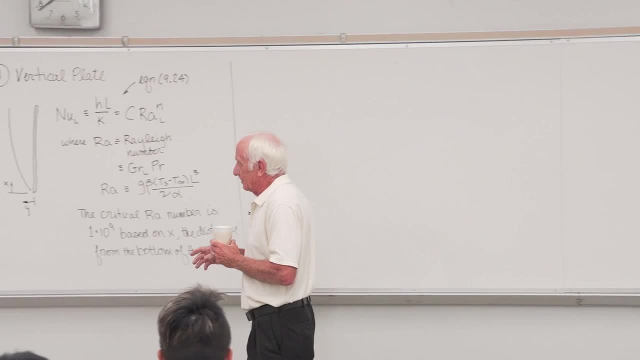 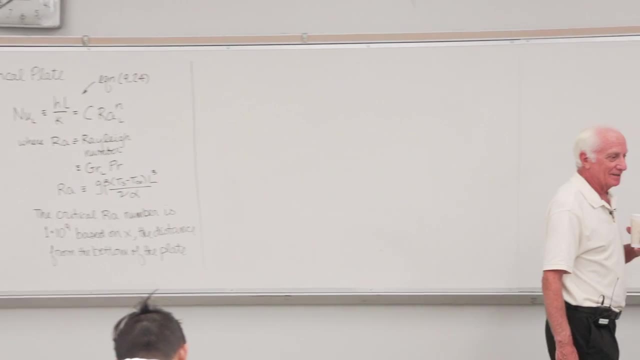 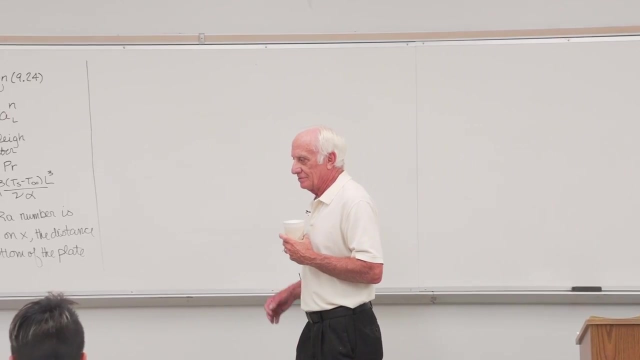 those vertical and horizontal cylinders are pipes and you know, go to any power plant, go to any manufacturing plant, there are tons of pipes. go to a solar collector field, there's tons of pipes. so we you deal with pipes tremendously. so there they are. they are important and we'll 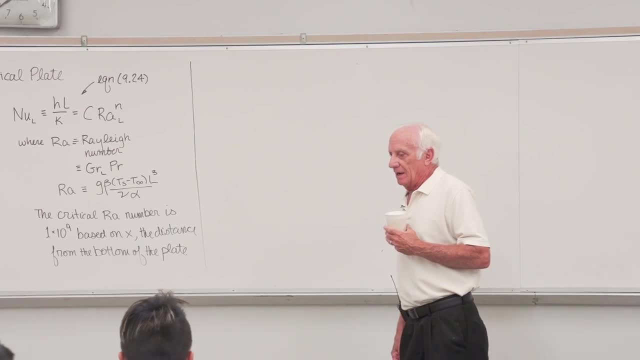 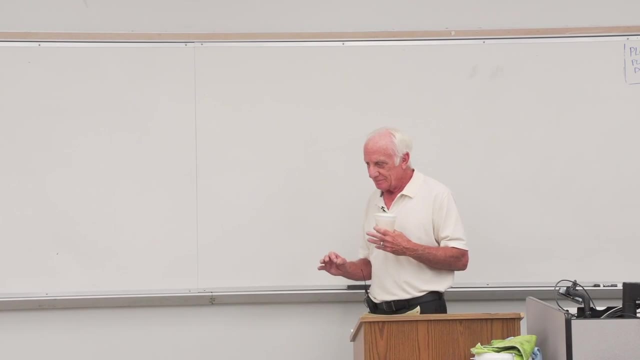 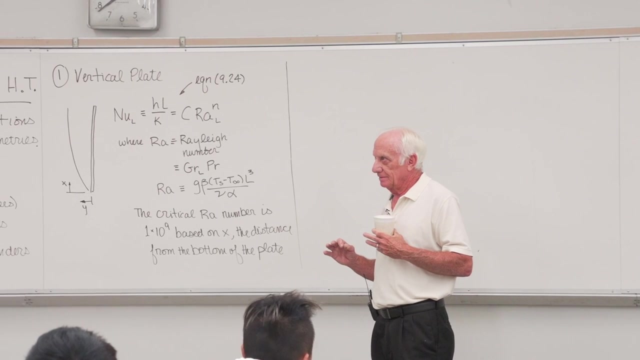 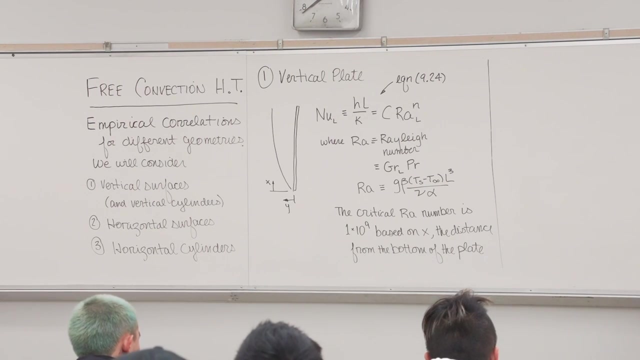 mention more examples as we work example problems now. just to remind you, there's no chapter 9 homework due to be turned in. this is the last chapter in the course, but I'm going to work in class at least four example problems using these geometries. in the textbook there are example problems- at least three good. 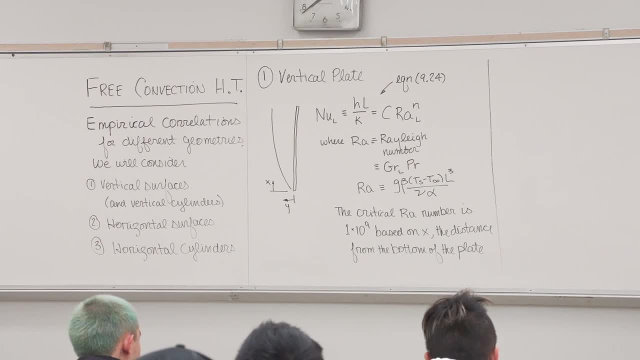 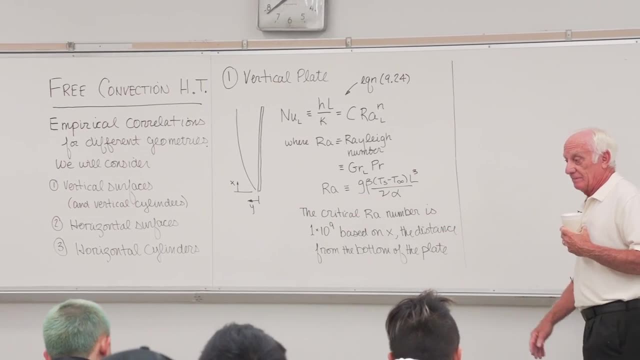 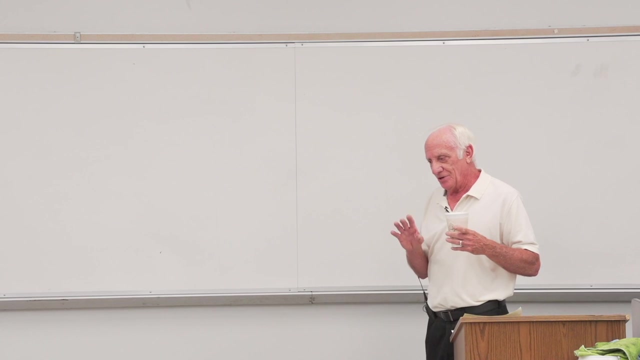 ones to look at. so you've got, you'll have roughly eight or nine example problems worked out for you, one of each of these guys and sometimes maybe two of a particular one. okay, so, just so, you look ahead and see what's gonna happen now. and, as you know, I mentioned that one of the problems on the on the final will 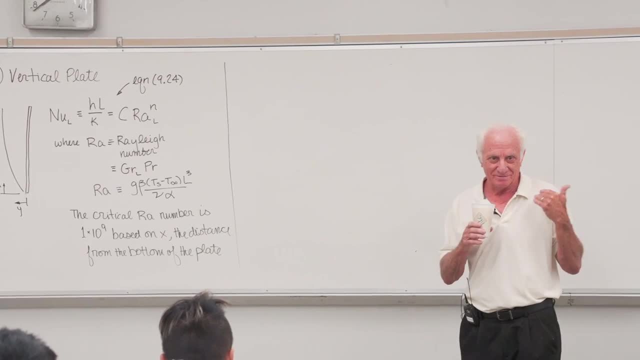 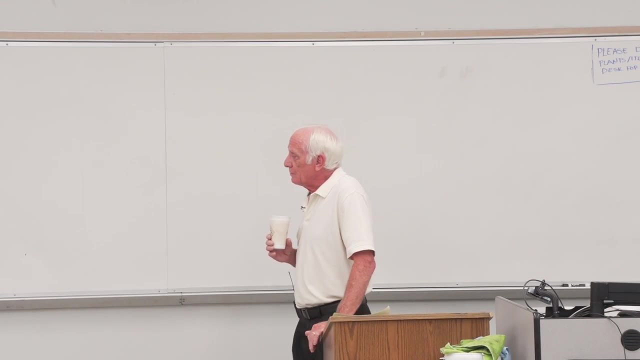 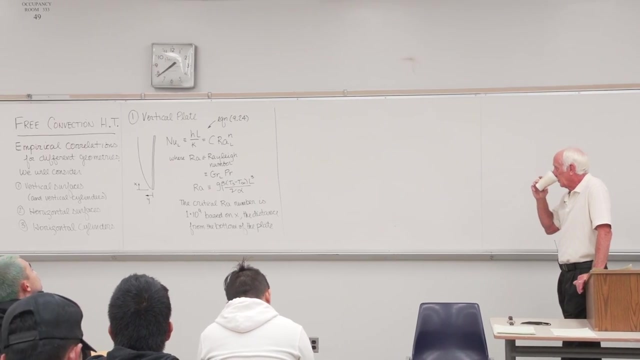 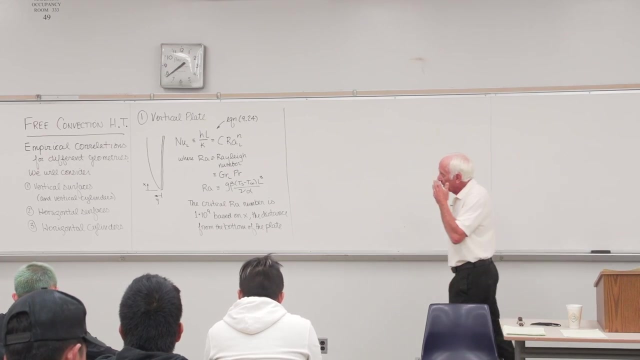 be chapter 9 problem. so 25% of the finals chapter 9. so you want to really make sure you're ready for that. okay, so we start out with a vertical plate, number one vertical plate. we looked at the picture the last time we met her, maybe two times ago. we drew the. 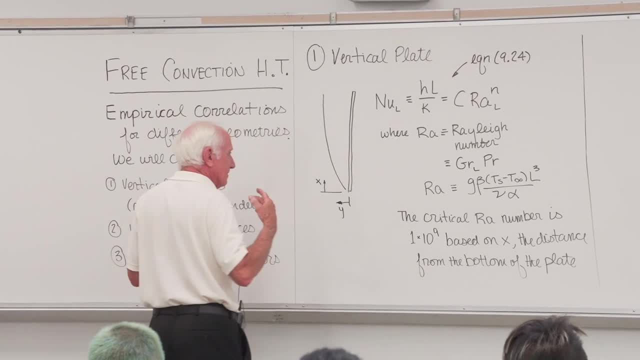 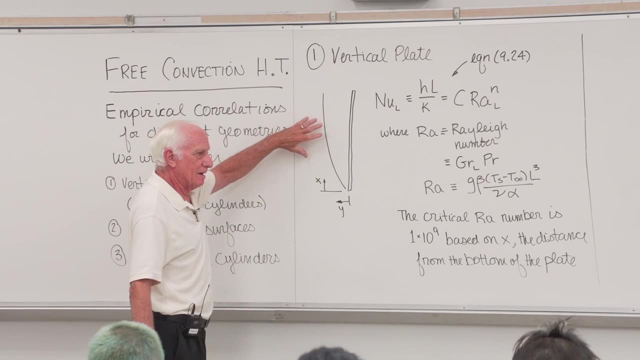 picture of what's going on. so let's just say the plate is being heated externally and the let's nothing. we just say it's air, for just to talking about it. the air outside so plates hot air is cold air touches plate, density goes down, voiancy effect. 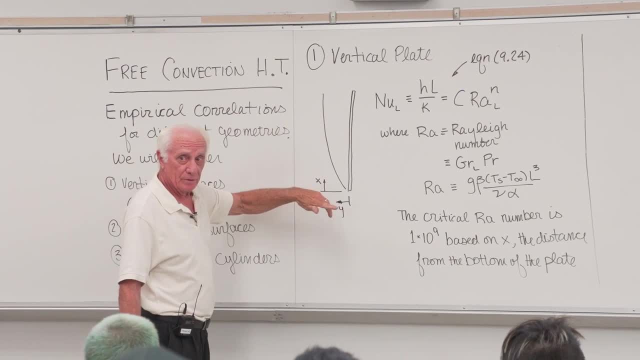 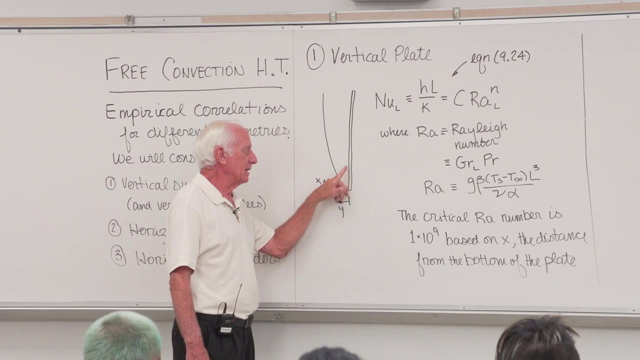 the air rises on the plate, a boundary layer builds up. from the leading edge of the plate down here, boundary layer builds up. we talked about that last time. we drew the pictures of how the temperature and velocity varied in the measure X along the plate length. length of the plate. this is L X equal L right. 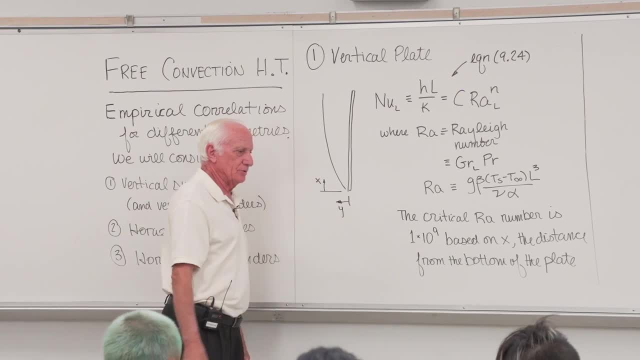 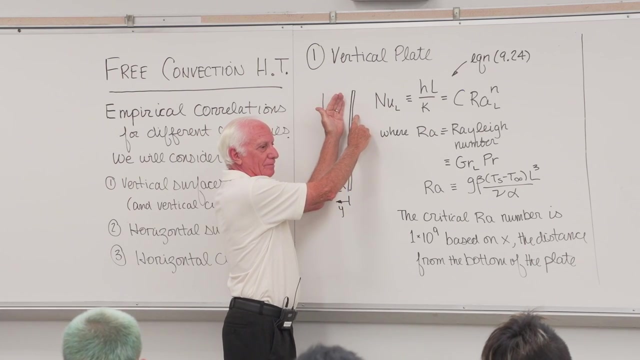 here Y is measured normal to the plate. so we did it, we did that last time and we done. by the way, if the plates cold and the air is warm, take this side over here. the air touches a cold plate, density goes up, it gets heavier, it drops. 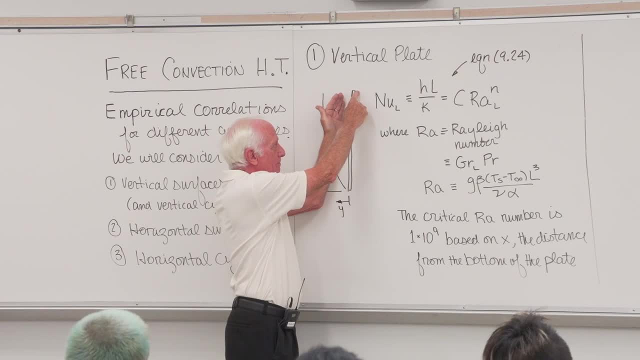 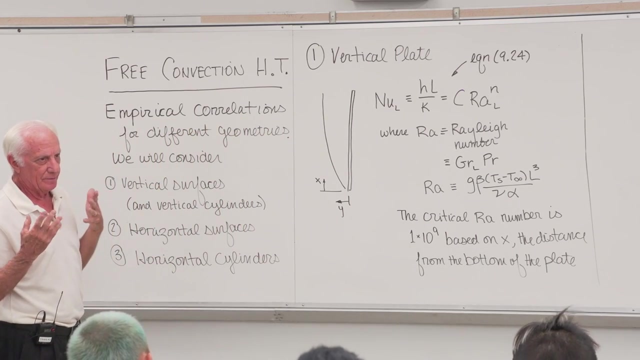 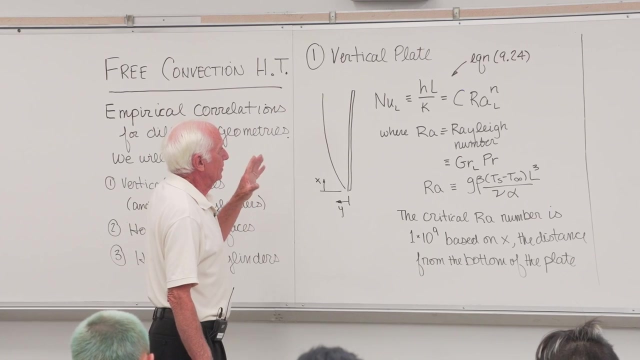 in that case, the boundary layer starts here at the top and it gets bigger as you go down. this is X equals zero. this is X equal L for the cold plate. okay, but we'll we'll pretty much talk about the surface being heated and the fluid being cooler as we go through this. we start out with the governing correlation. 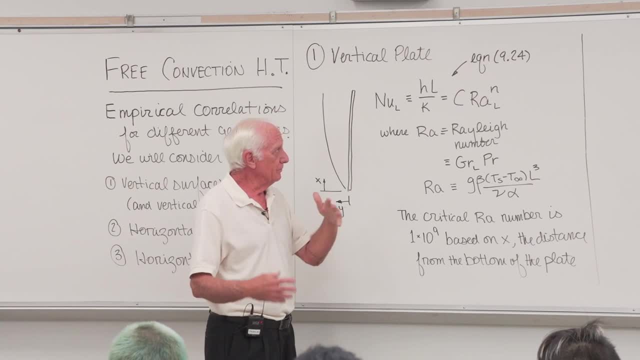 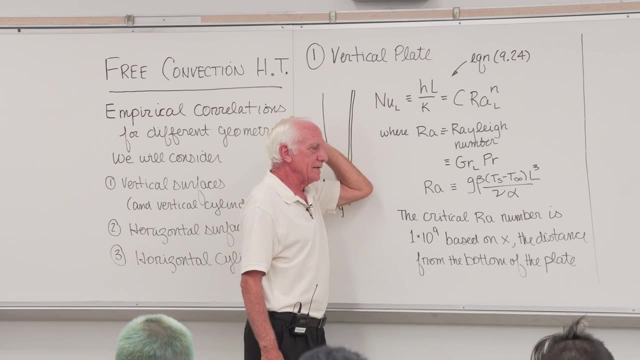 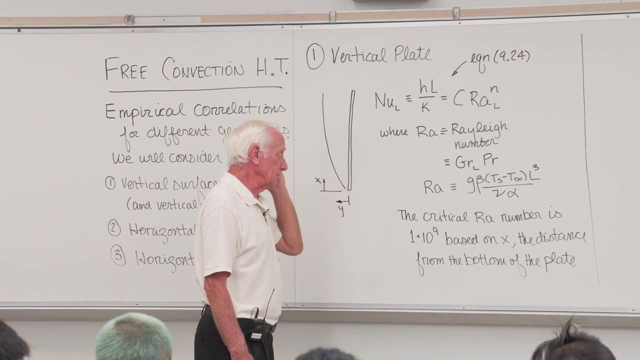 equation, which is again the no salt number. you know salt based on length, L, don't forget this- is L H, L over K. it's equal to a constant Rayleigh number: L to the end, now the Rayleigh number. the Rayleigh number is a dimensionless parameter, as I said before. you know tons of them in. 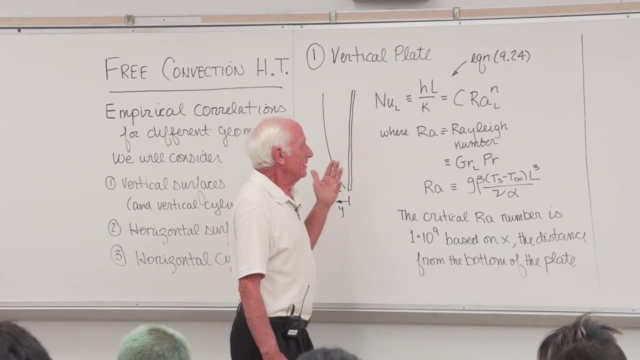 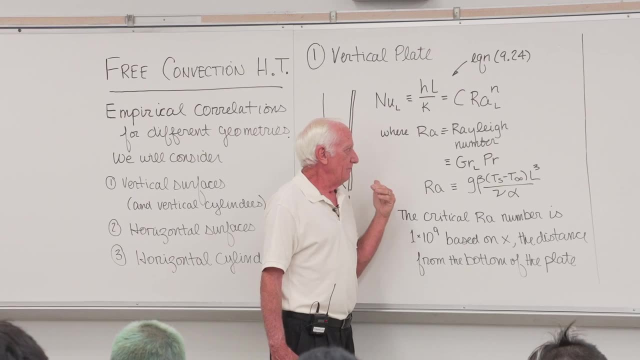 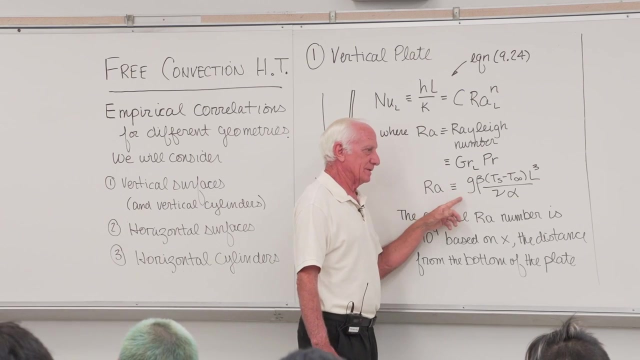 convection, tons of them in convection. the Rayleigh number is the Grashof number times a. Prandtl number two, dimensionless numbers two. that's the only dimensionless property of the fluid we know. we got the grass shelf number in our previous lecture. so if you multiply grass scenarioord, this guy 저희. 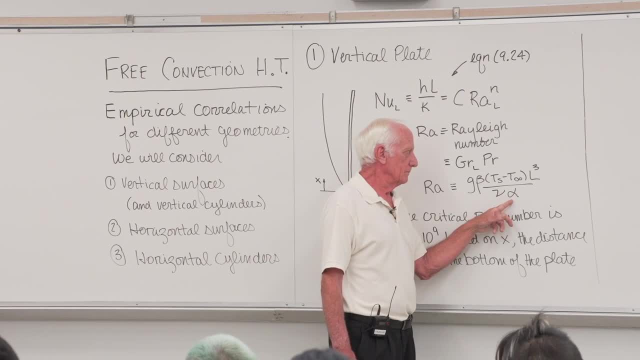 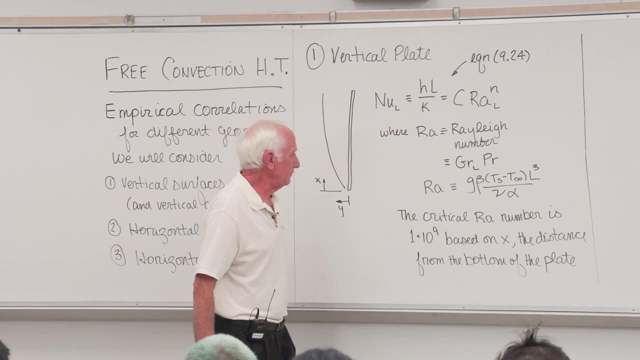 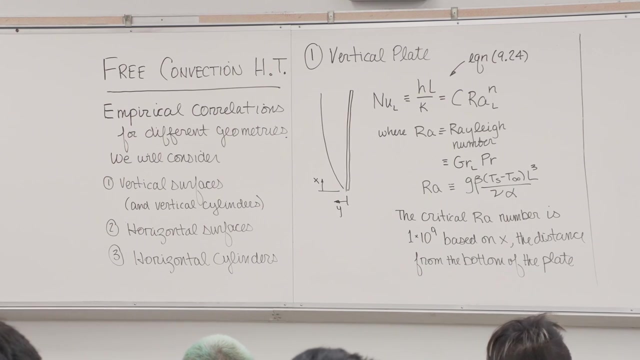 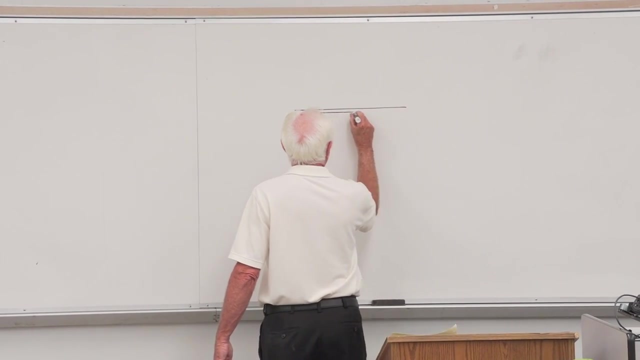 magnetic viscosity divided by thermal diffusivity times, L, cubed L height of the plate over here. Now, if we contrast that plate to Chapter 7, here's Chapter 7. We could have all laminar flow or we could have mixed flow. 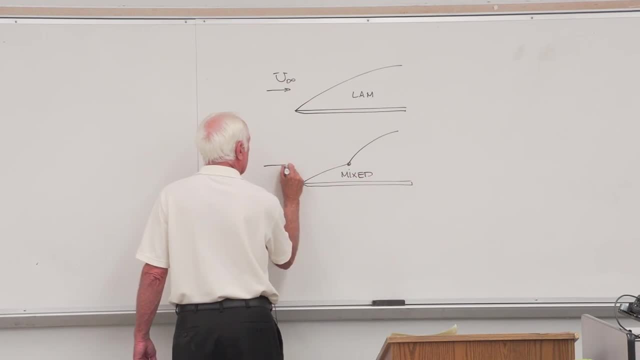 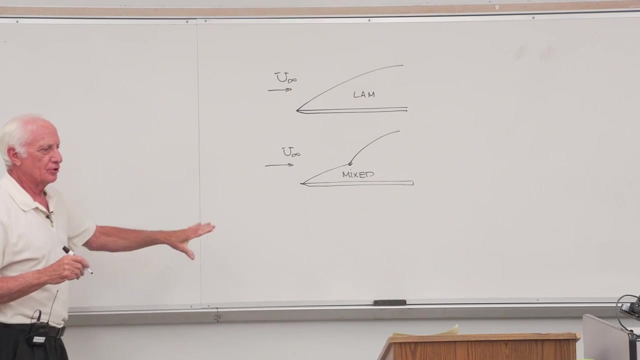 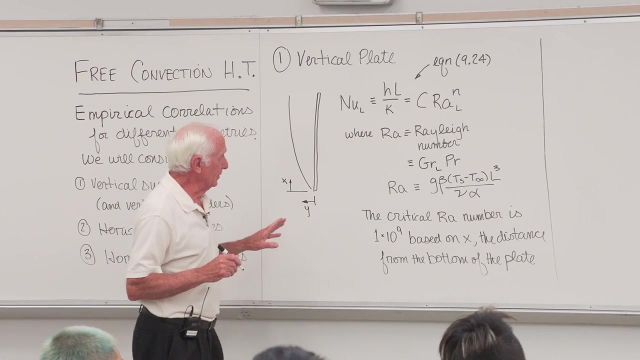 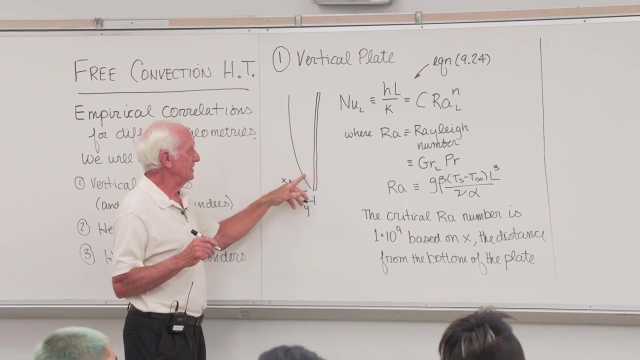 part laminar, part turbulent. Chapter 7, we had an H equation for each This case, this case and even a third case all turbulent Over. here we have the possibility of an all laminar boundary layer, or maybe the flow transists at some x-value to turbulent. 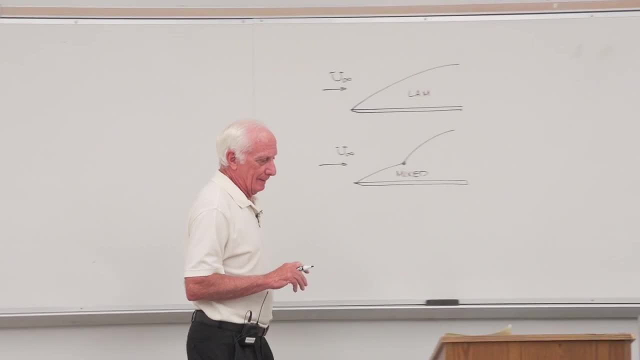 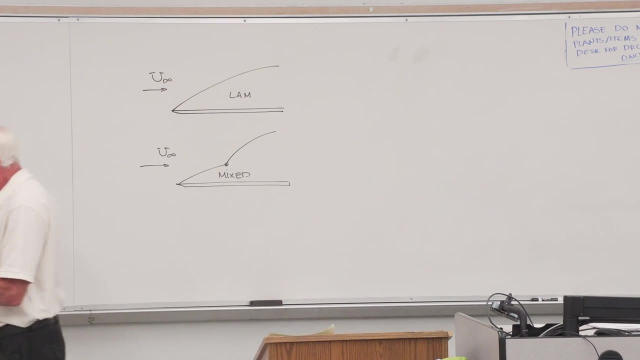 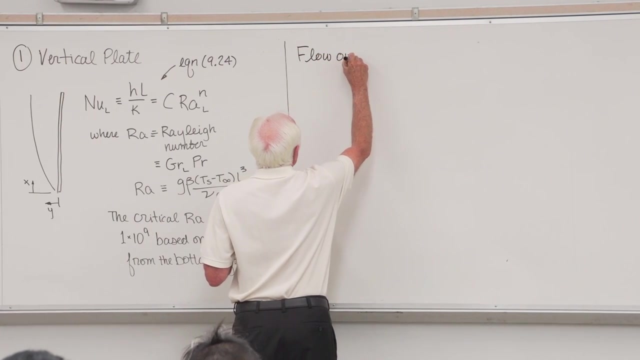 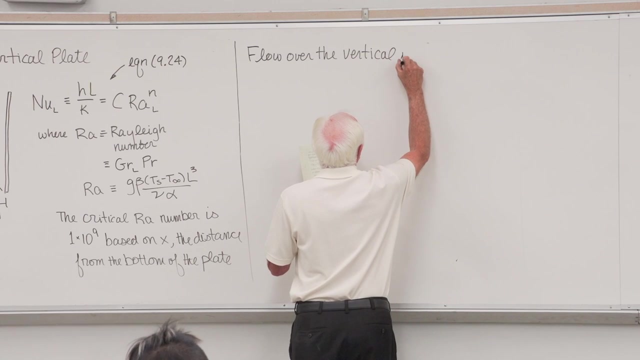 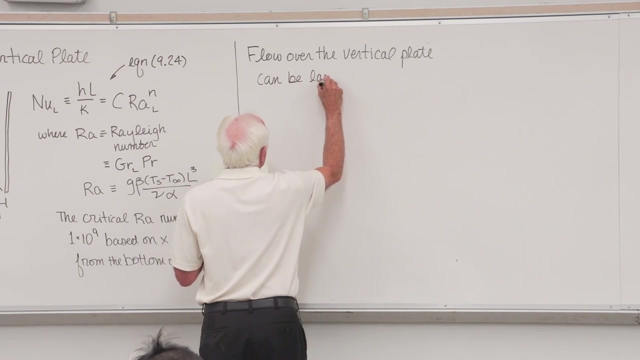 so we have a mixed flow region. So we have to look at that. So let's take a look over here. then Flow over the vertical plate can be laminar or turbulent. In other words, it can transist at some x-value to turbulent. 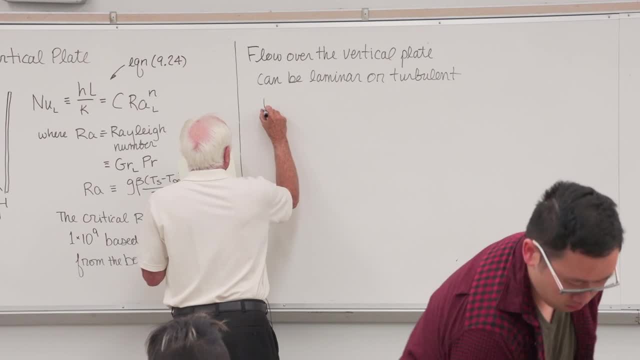 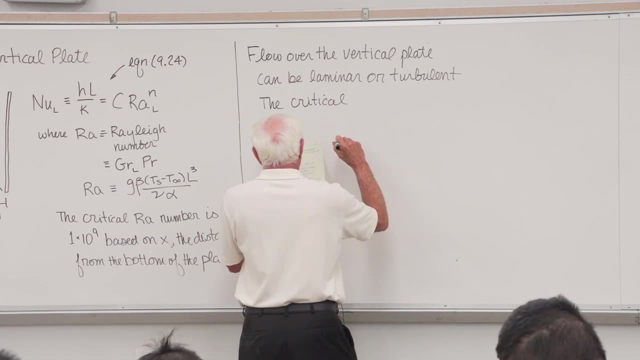 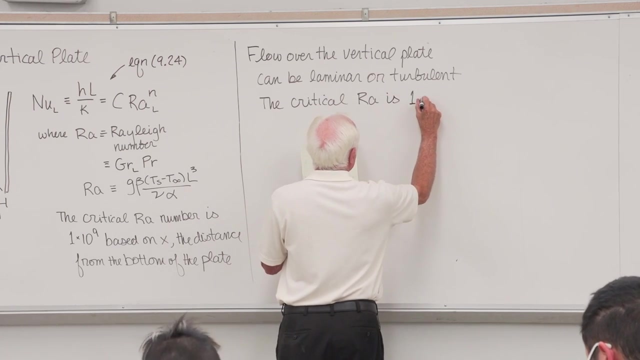 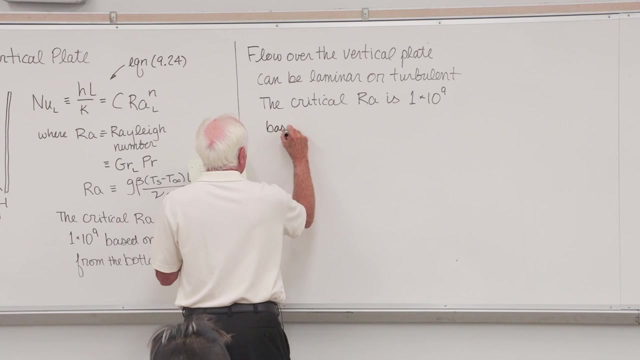 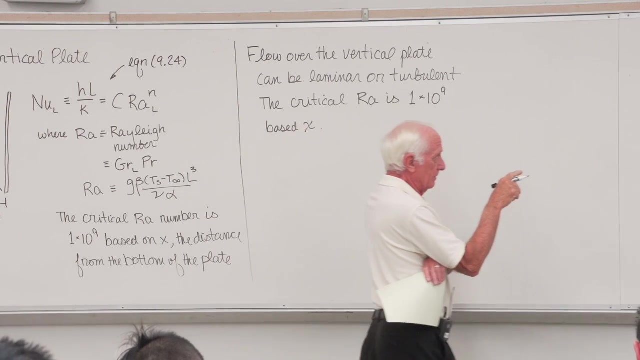 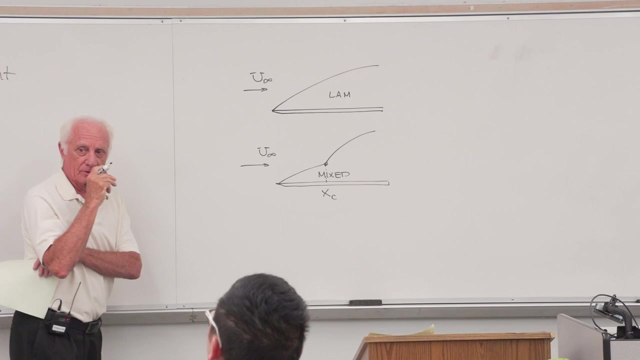 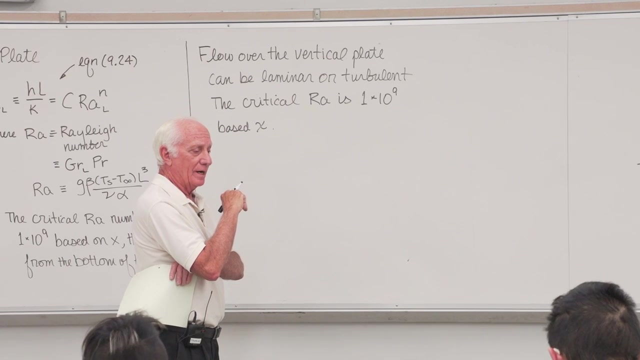 a turbulent boundary layer. The critical Rayleigh number is 1 times 10 to the ninth, based on x. Let's go back over here to Chapter 7.. That was x critical in Chapter 7.. We could find that. Why The magic Reynolds number for flow over a flat plate? 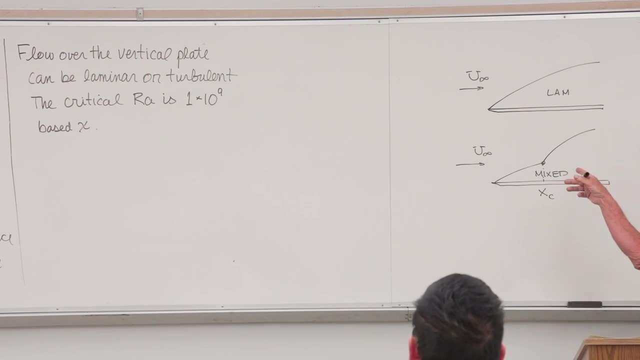 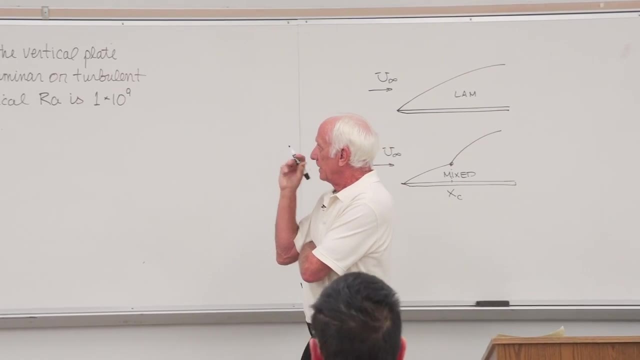 5 times 10 to the fifth, So I can find x sub c for this problem. Once I decide it's turbulent here, I can find x sub c Over here, different. This is a Rayleigh number. What's the magic number? 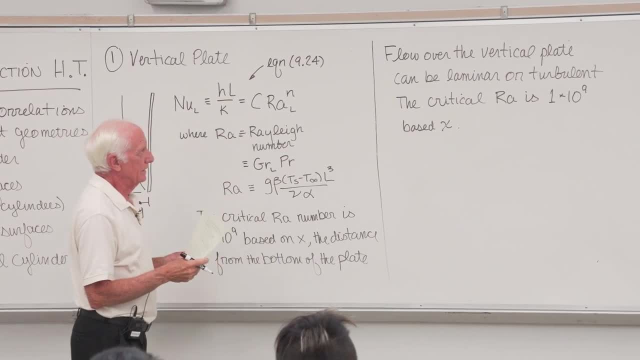 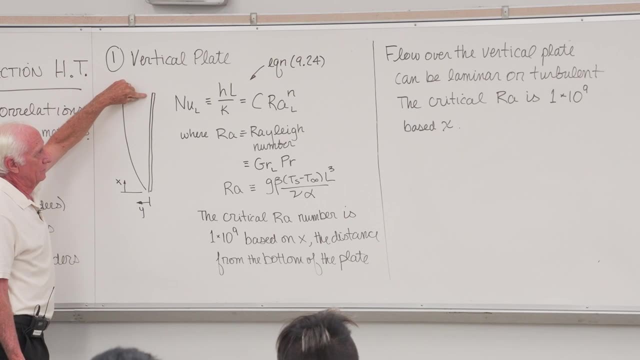 1 times 10 to the ninth. If the Rayleigh number here 1 times 10 to the eighth, it's all laminar. If the Rayleigh here is 1 times 10 to the eleventh, it's laminar turbulent. 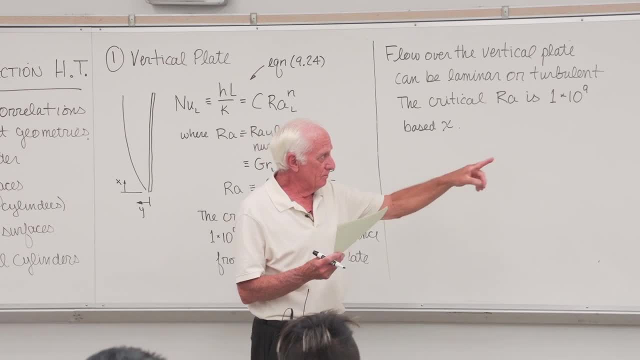 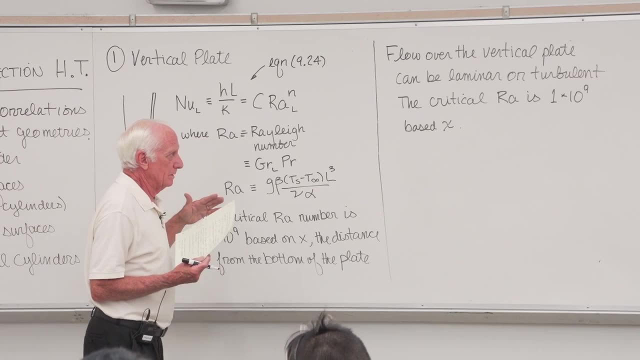 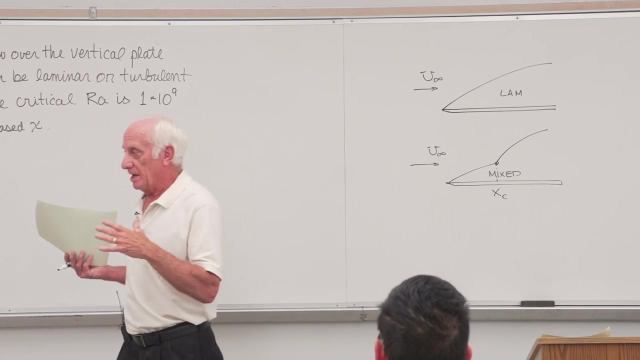 Same but the same method, just like in Chapter 7, the same method of doing this. And, by the way, in Chapter 7, everything is dependent on the Reynolds number. In Chapter 9, you're never gonna see the Reynolds number. 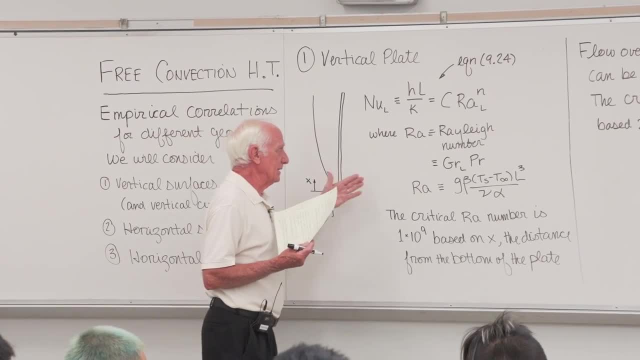 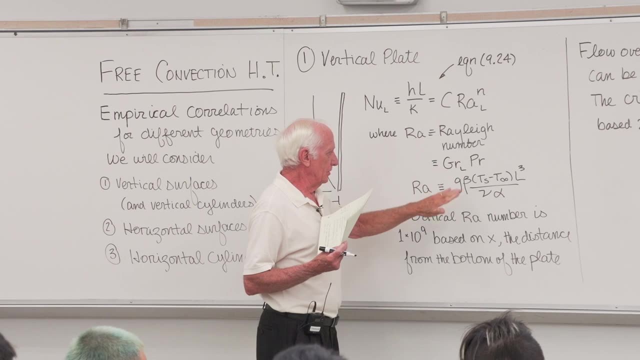 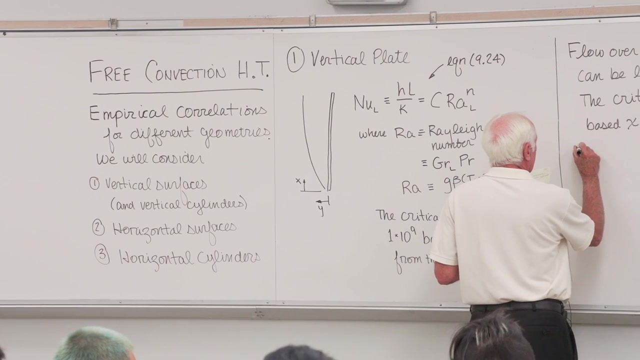 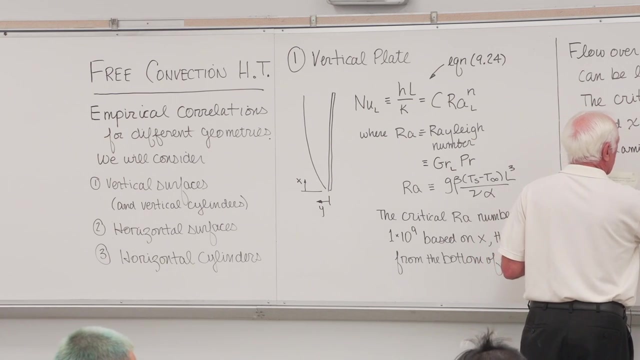 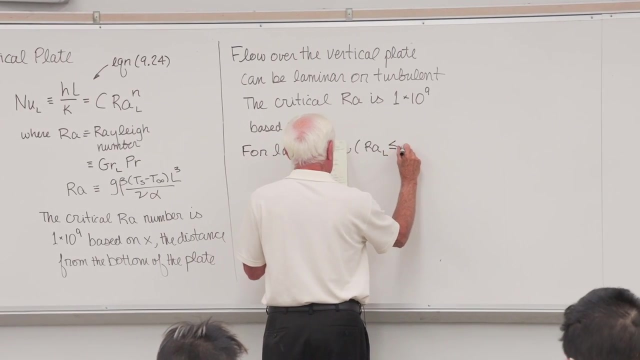 In Chapter 9. now the magic, dimensionless parameter is the Rayleigh number. All the equations have the Rayleigh number in them. Laminar turbulent has the Rayleigh number in it. So for laminar flow, Rayleigh number based on L less than 10 to the ninth. 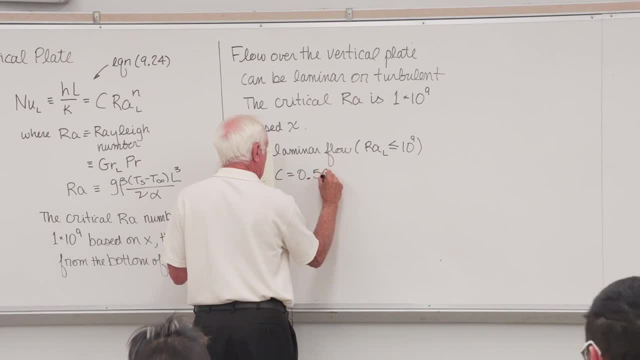 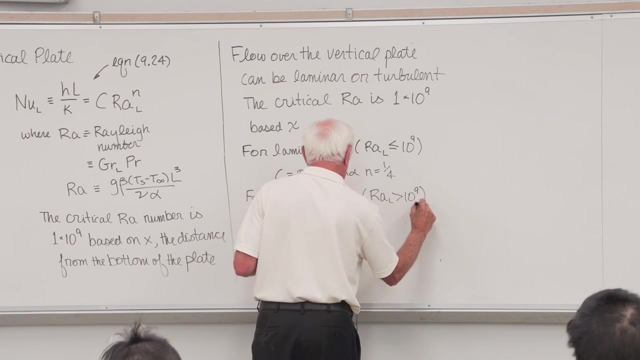 Values of c perqueeds plus F for one time. plus F plus E is something like this. Thanks for watching. See you next time. Turbulent flow: we have part laminar, part turbulent. Rayleigh number is greater than 10 to the ninth. 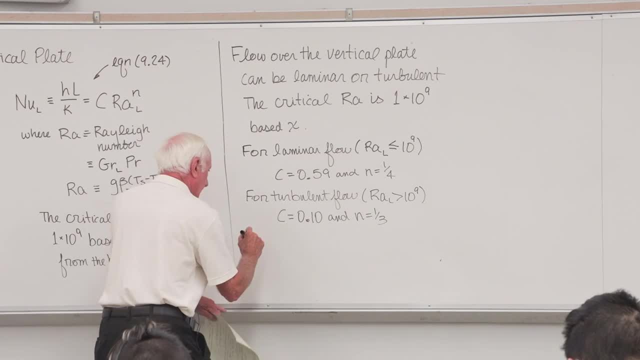 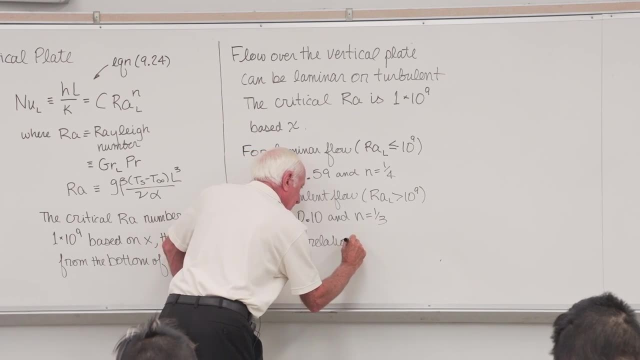 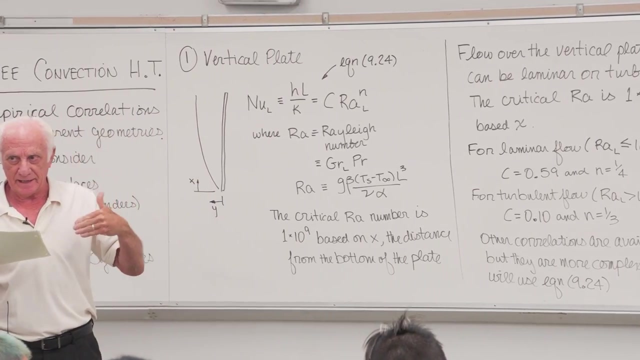 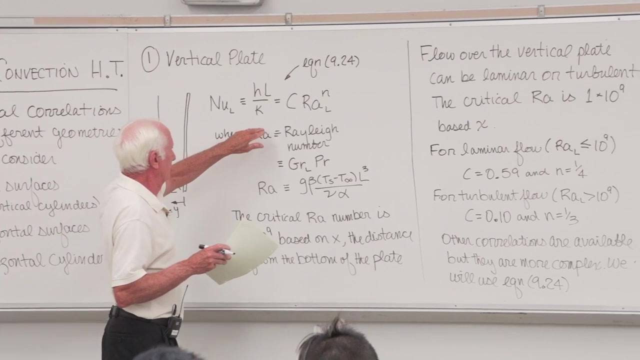 Thank you. Now, of course, there's different correlation equations available. This one is an earlier one, which might not be as accurate or good over a range of values as other ones, So there are other correlations available that you would probably use rather than this one. 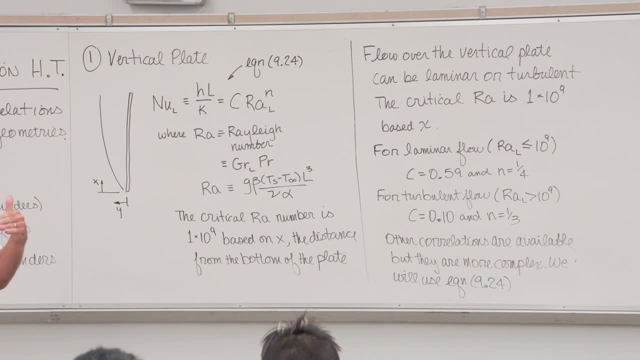 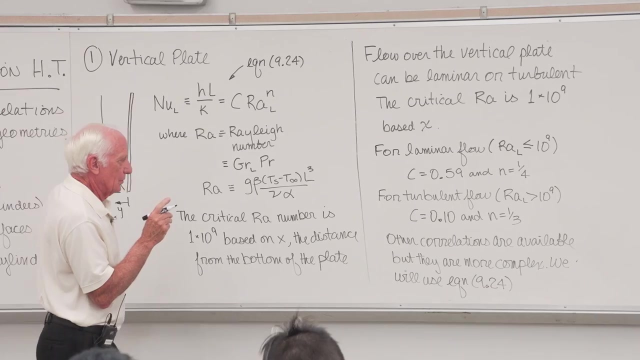 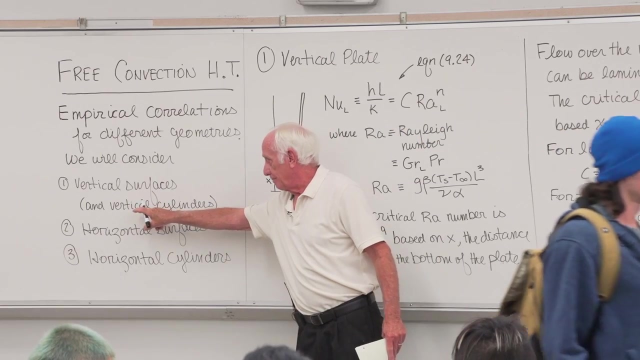 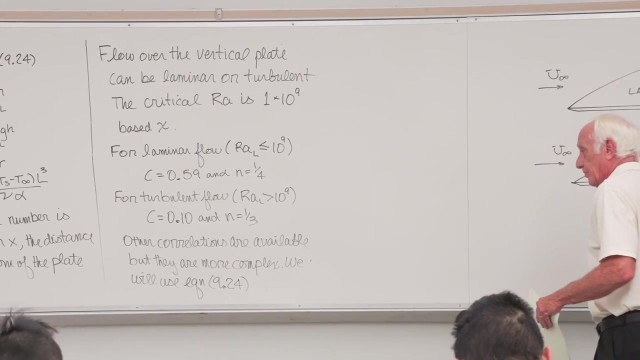 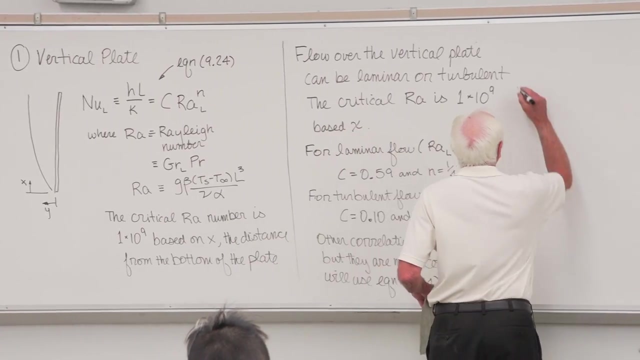 But for the purpose of our class and the textbook and so on, we're going to use this one 924.. This vertical surfaces- it says here parentheses- and vertical cylinders. Okay, You can use this also for vertical cylinders sometimes. Okay, I think I'll put that up here. 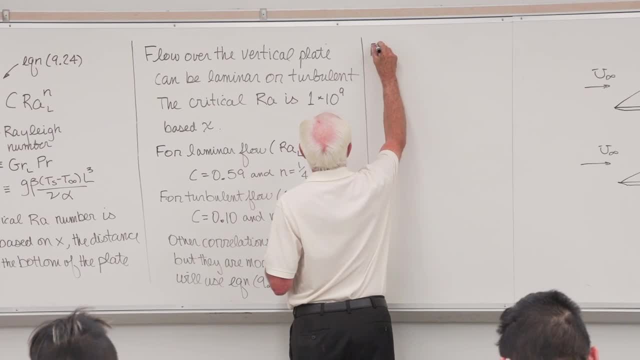 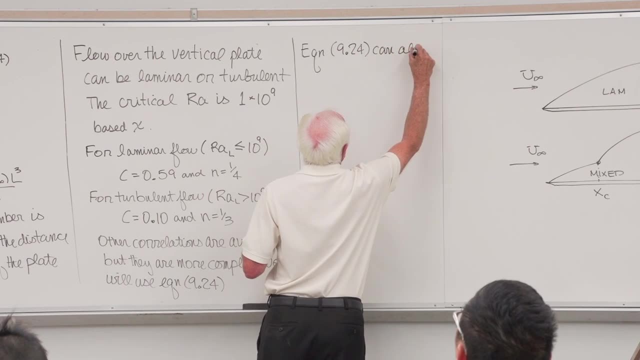 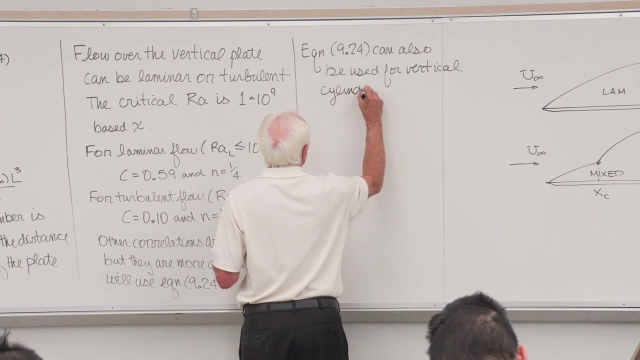 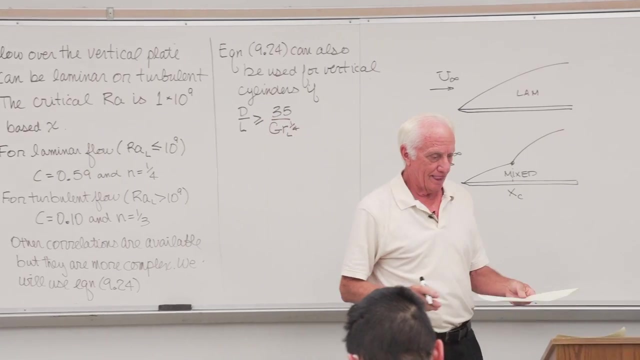 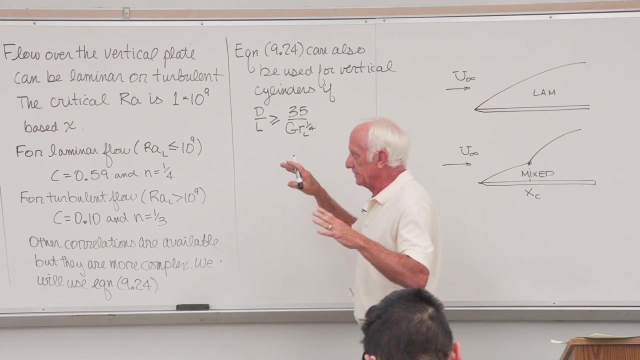 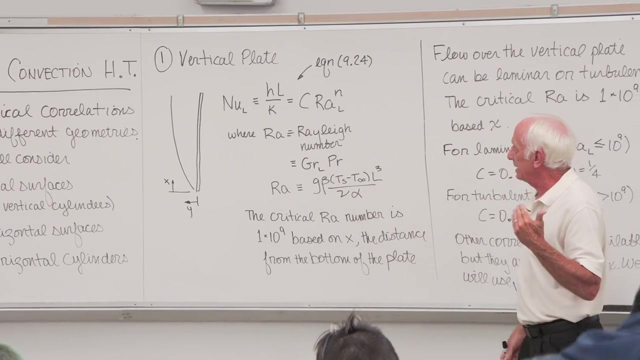 So equation 924.. But this has to be satisfied. Before I describe this equation, let me back up a bit and say all this stuff here. this equation is based on empirical correlation. What does that mean? That means somebody took a vertical surface out in a lab. 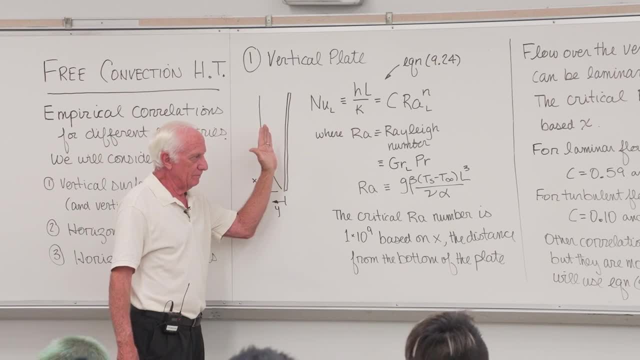 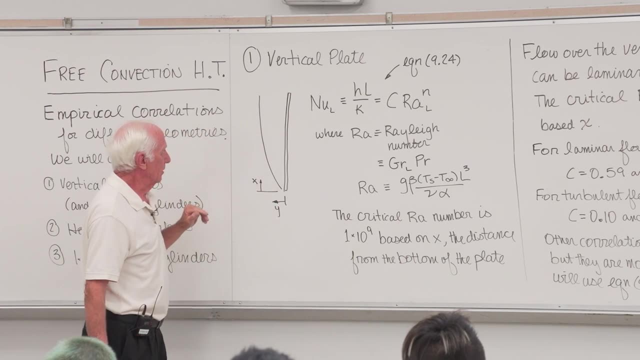 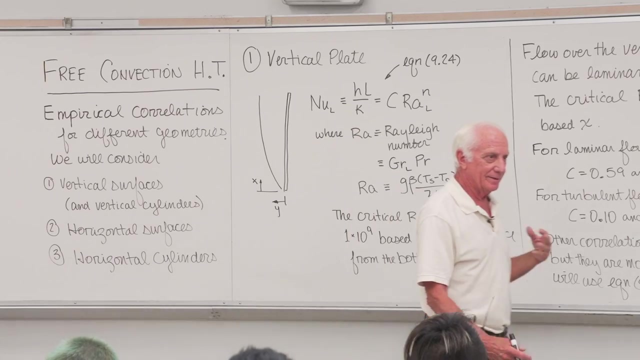 They heated it with a power supply. They knew how many watts went into the power supply. They insulate the backside and the sides of the plate. All the heat goes out to the- let's say it's air. You equate that to H A, Delta T and you solve for H. 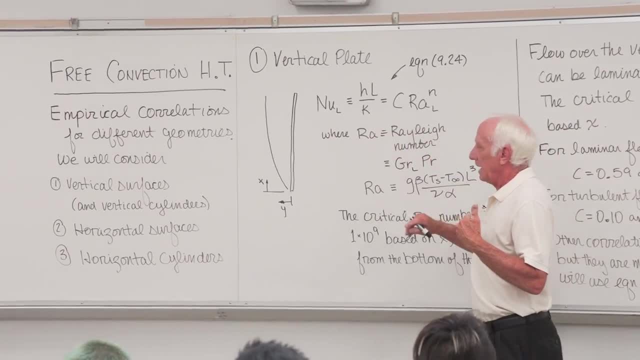 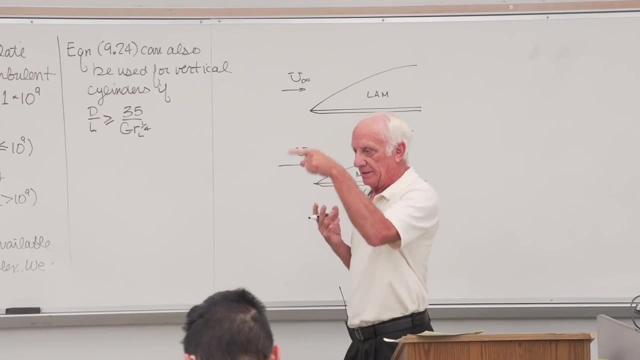 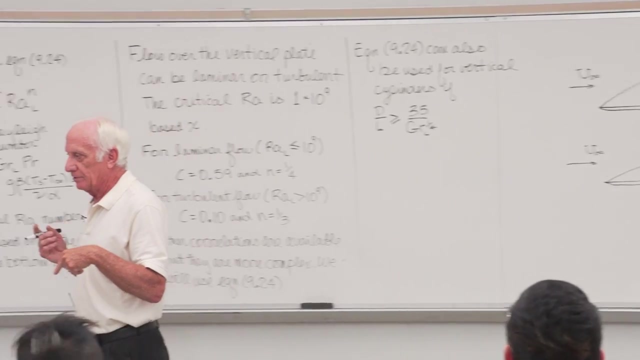 Knowing H you get the Nusselt number. Then you correlate the data from probably some plots of dimensionless parameters: Nusselt on the y-axis, Rayleigh number on the x-axis. We did that for circular cylinders in Chapter 7.. 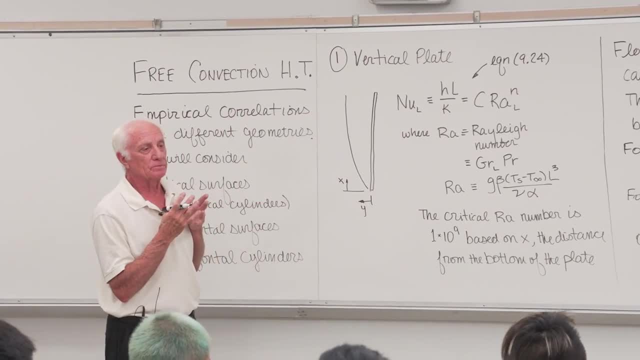 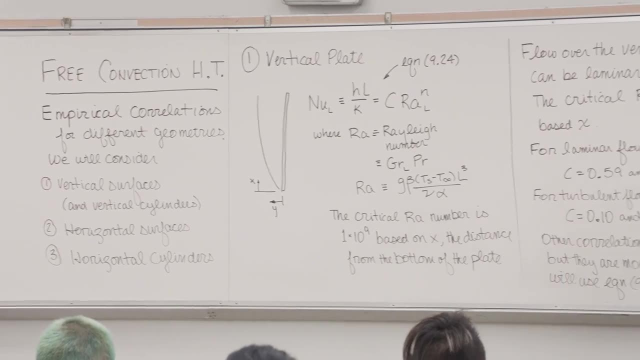 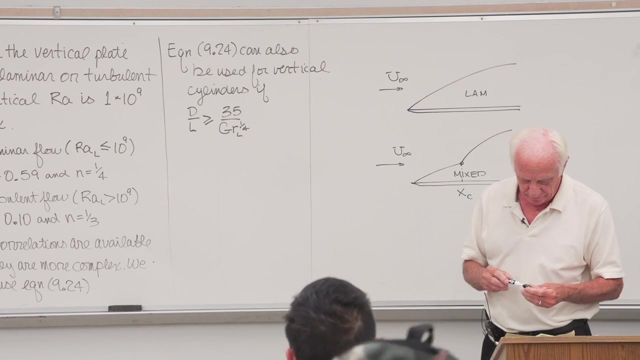 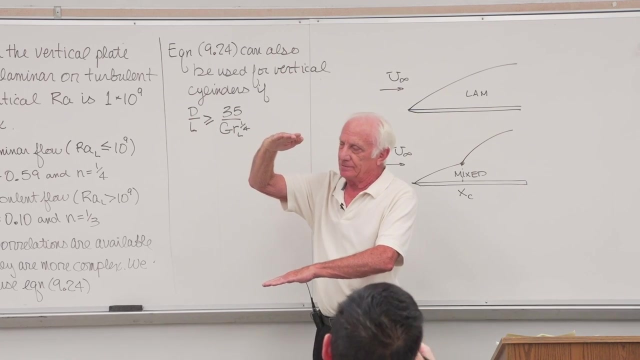 Anyway, it's done in a laboratory environment. experimental Data was taken and these constants then come from those experimental observations. So if you take the diameter of the cylinder divided by the length, which is the height of the cylinder, L greater than 35 over Grashof. 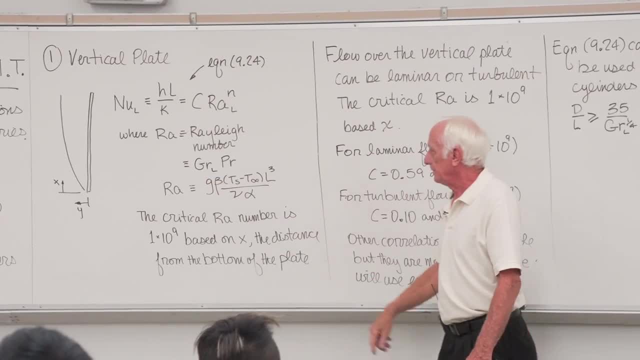 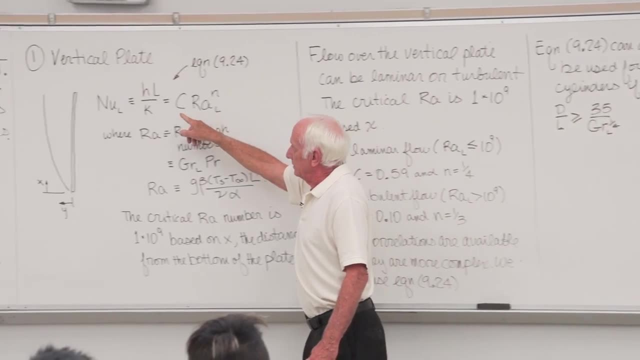 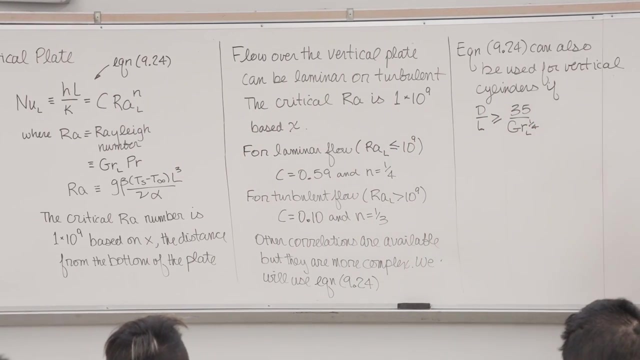 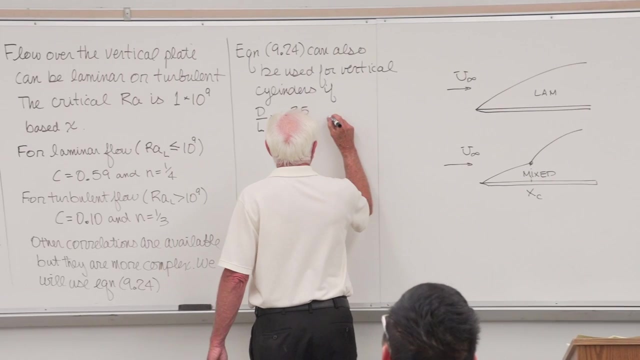 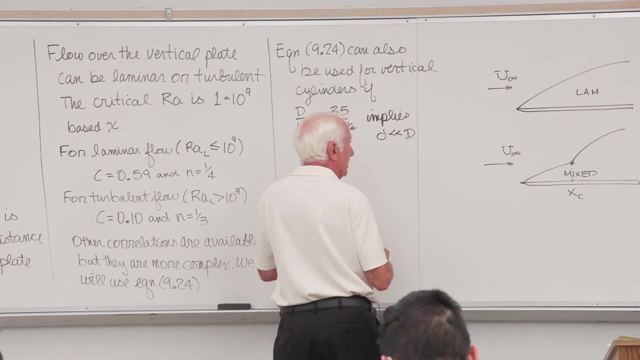 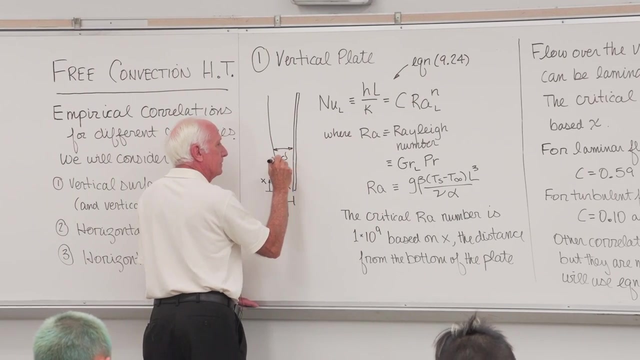 Grashof is in your notes from last time Grashof. Then you can use this equation to find H for vertical cylinders, And the textbook says what this implies: Delta is much less than diameter. Delta is the boundary layer thickness. Delta is the boundary layer thickness. 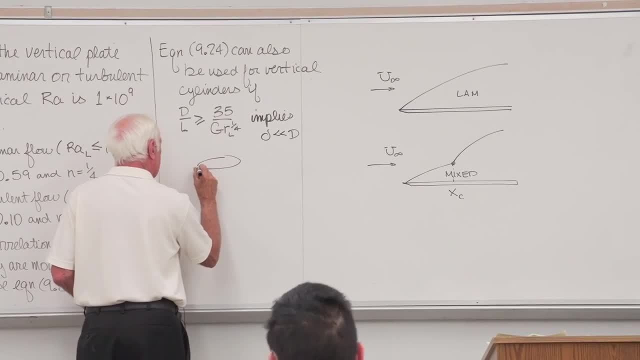 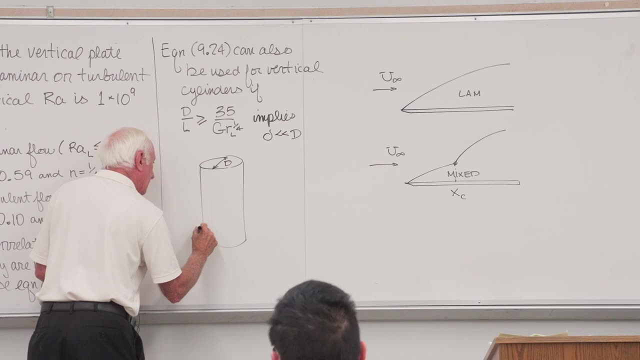 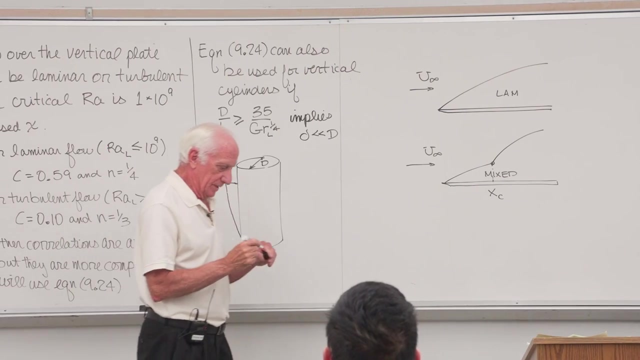 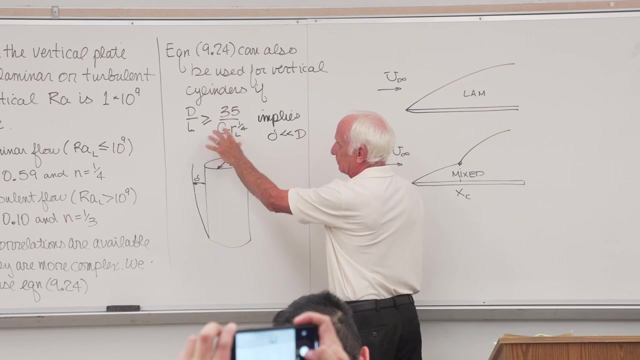 Delta is the boundary layer. thickness Boundary layer builds up, that's delta. If delta is much, much less than this diameter, That's what this thing really implies. But you calculate this guy and if that's true, you can use that equation. 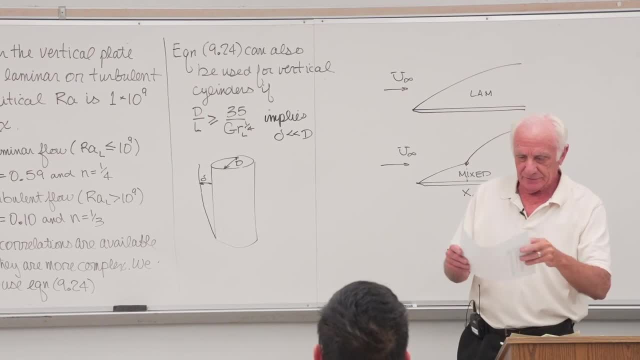 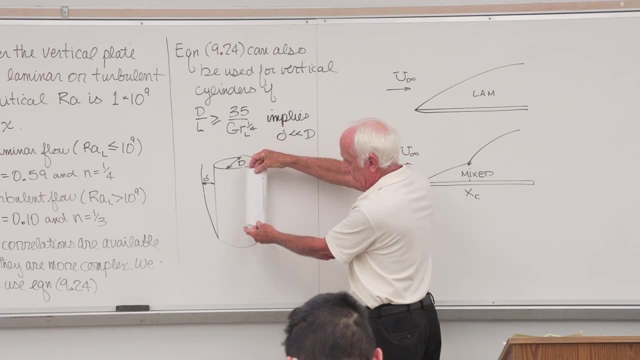 Okay, See, there's the vertical cylinder, It's got a diameter. A boundary layer builds up from the bottom and it goes up. This equation, if it satisfies, implies that the boundary layer thickness delta is a lot less than the diameter. 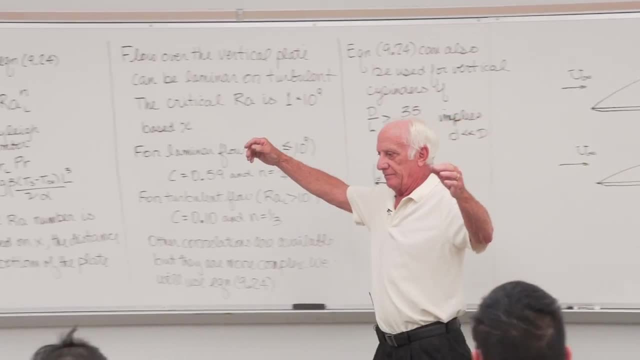 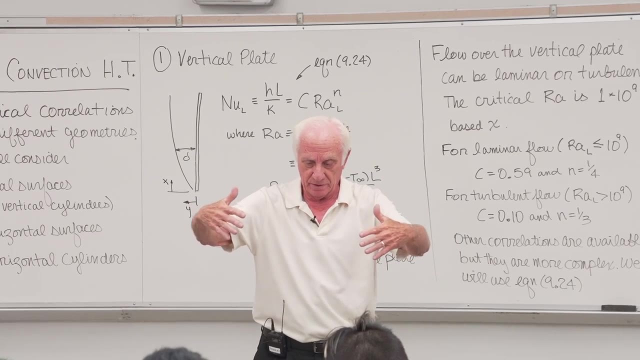 For instance, let's say you had a three-foot diameter tank of oil and you're looking at the outside, the tank is warm because the oil is warm. So the outside the tank, three-foot in diameter of hot oil, a boundary layer builds up in the air. 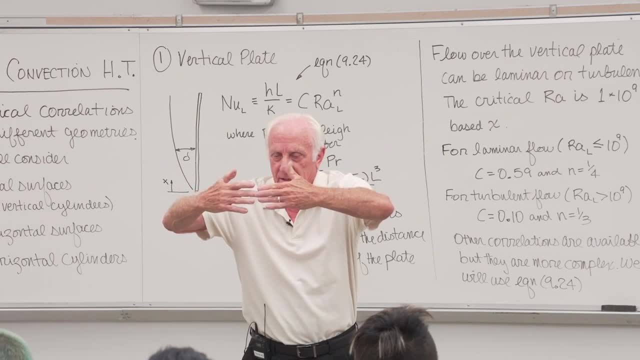 If I look at the outside that tank in a certain angle, let's say 10 degrees, whatever does that surface of tank almost look like a vertical plane wall. Yes, it does, Yes, it does. These two hands are almost formed. 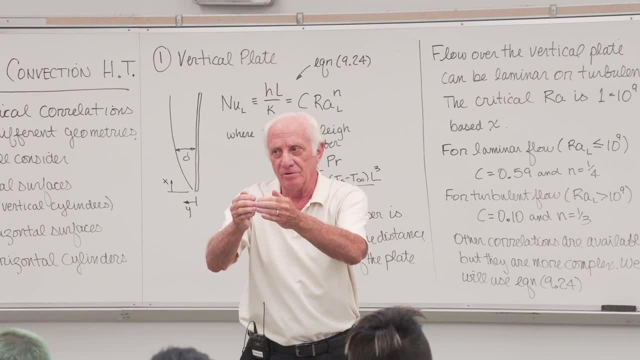 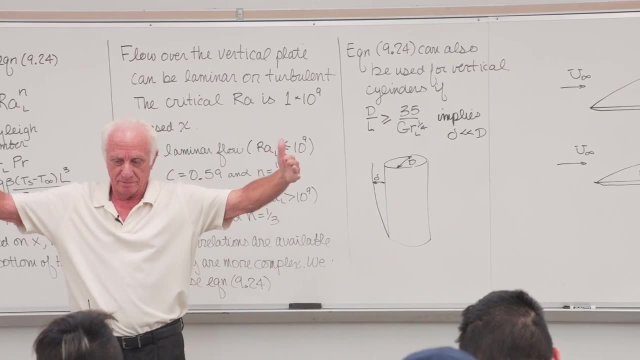 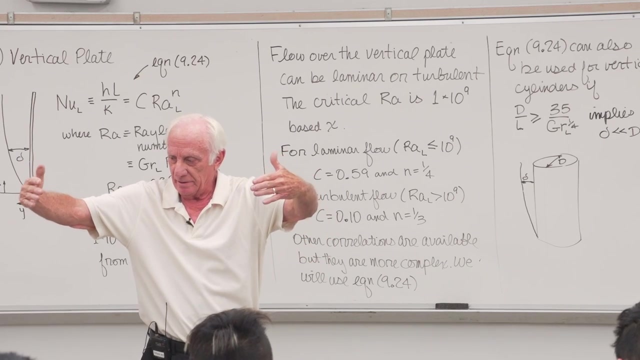 a vertical. Now make a small cylinder. Now is it a plane wall? No, no, no, uh-uh. So this D, if it's real big, then typically delta is small compared to the diameter of the tank. 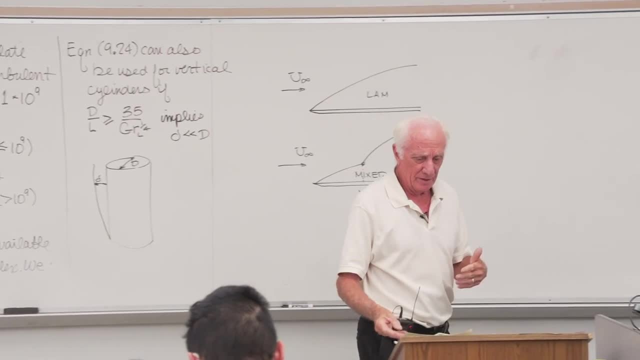 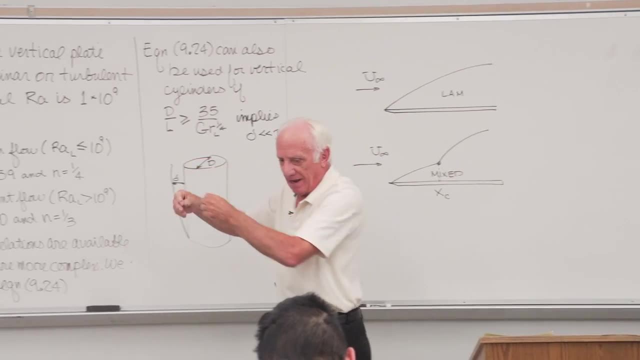 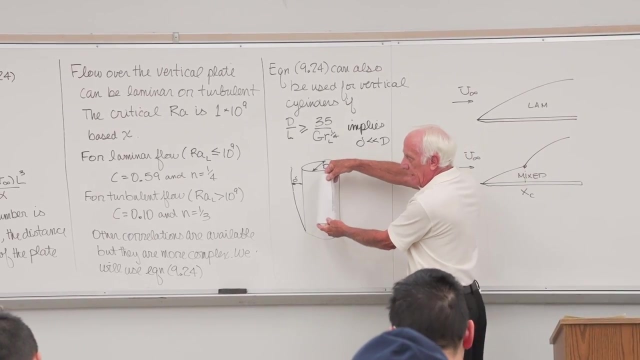 So just walking through it- from a physical point of view, that's what it means. You can approximate the wall of the tank as being a plane wall. unwrap it, You take the cylinder and you unwrap it and it looks like a plane wall, like that. 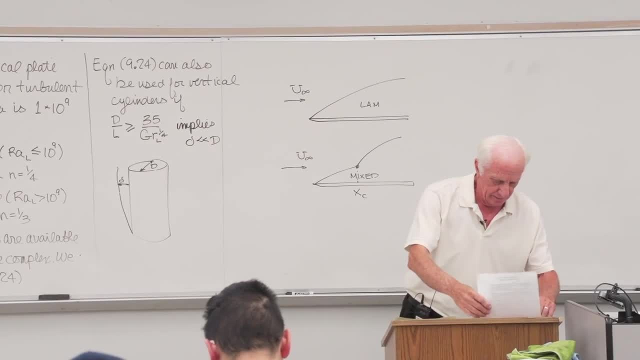 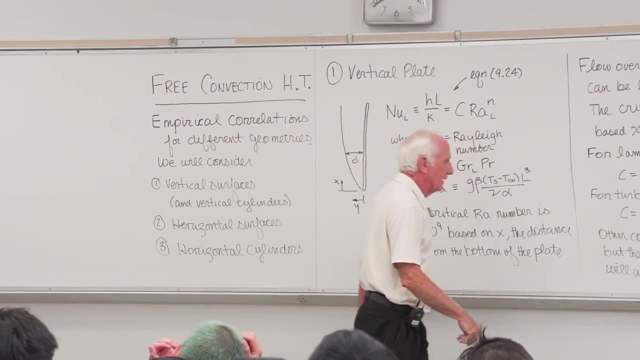 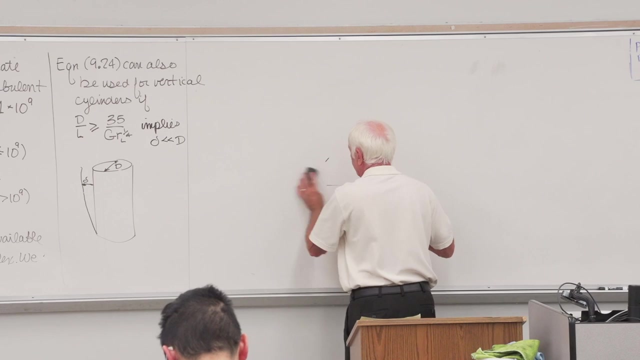 That's what it's doing, Okay, so now we've covered one: vertical surface, vertical cylinders. okay, Let's take a look at the next one. We're going to jump to three, because three is easier than two. Two is the toughest one. 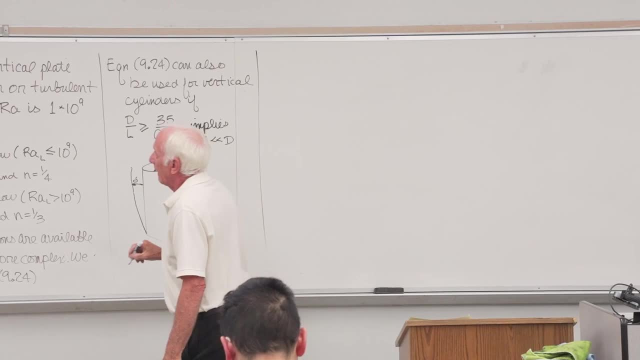 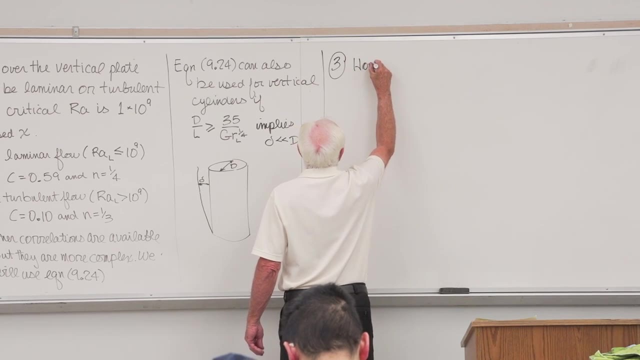 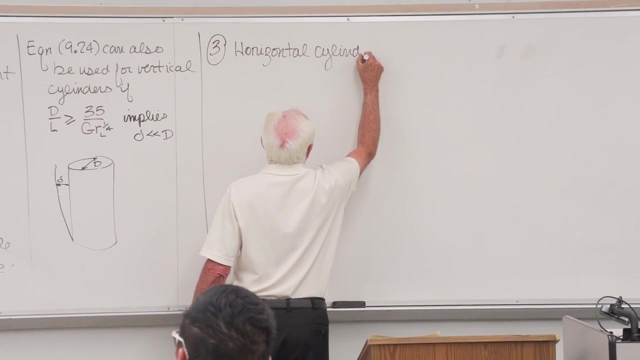 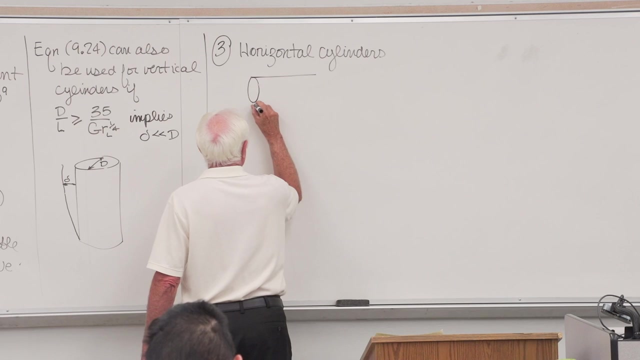 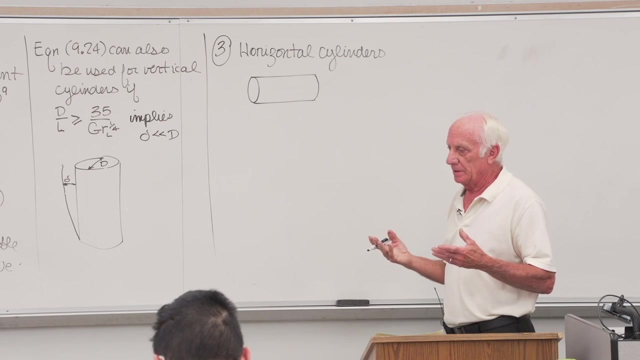 So let's look at three. Three is horizontal cylinders. Okay, Now of course we're looking at geometries like this. Of course, if the cylinder is hot and the fluid is cold, air is colder, then heat's rising off the cylinder, or vice versa. 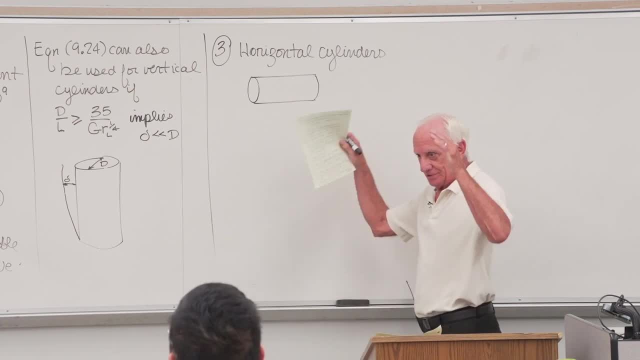 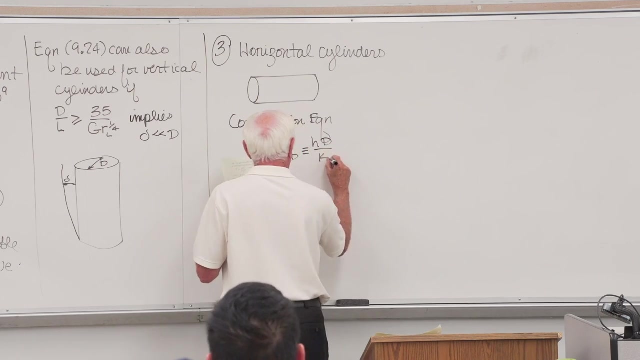 The cylinder is cold and the air is hot, and it just works the other way around. Here's the correlation equation. So the air is hot, the fluid is cold and the air is hot. Now we're looking at the diameter of the cylinder. 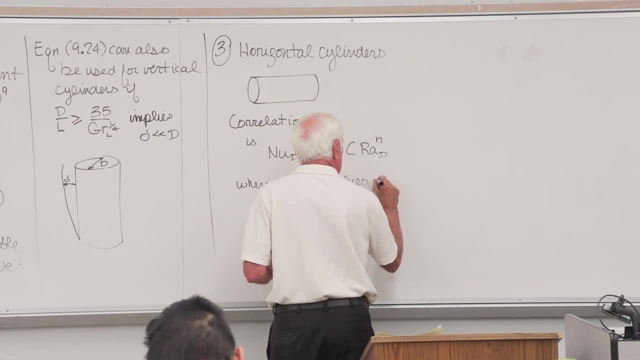 the diameter of the cylinder, and you can see here that diameter is important, Not L length. Diameter is the important dimension. The CNN values depend on the Rayleigh number. The C and N values are the same. The C and N values are the same. 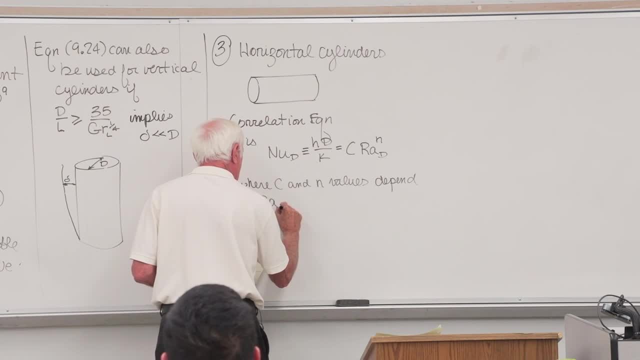 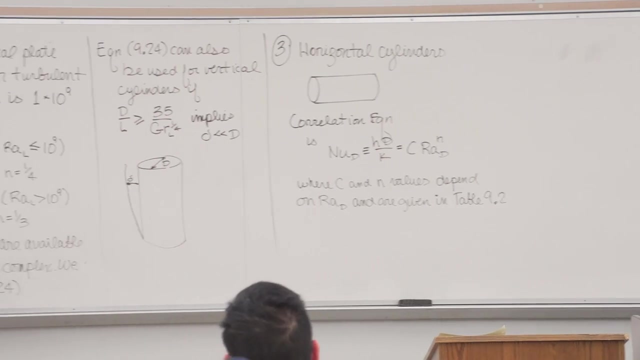 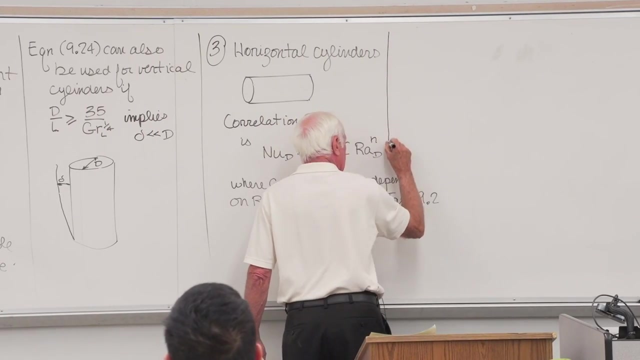 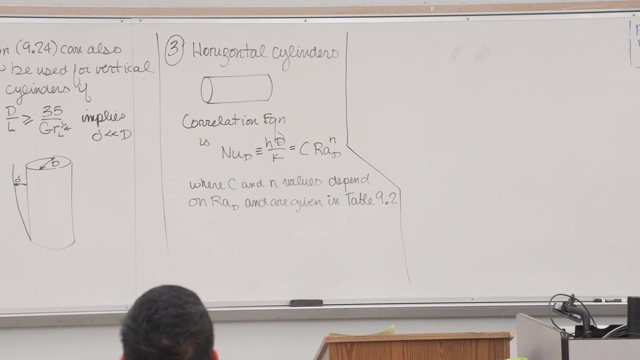 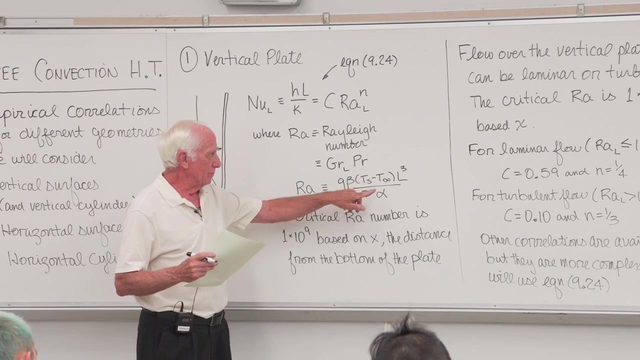 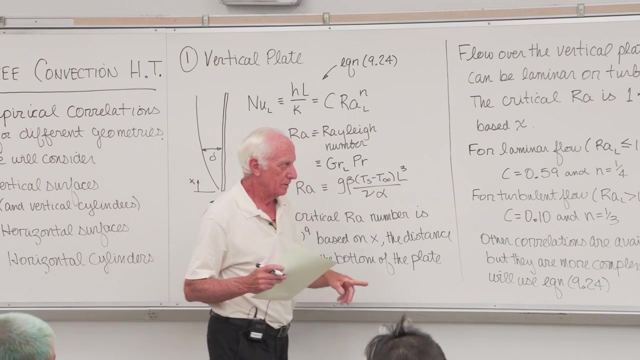 Table 9-2, so it's very straightforward. There's only one equation: Rayleigh d. it's like a Rayleigh here. Rayleigh, subscript d replaced the L with a d, so Rayleigh d has d cubed here in the equation. 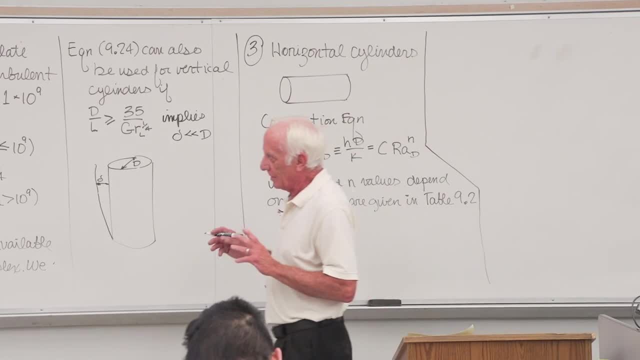 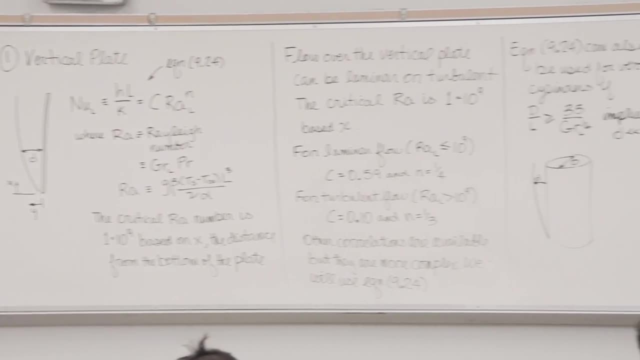 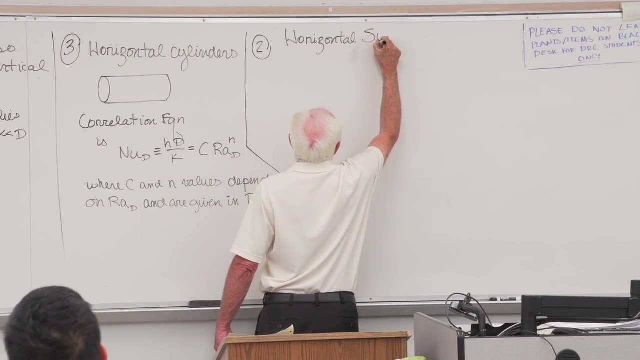 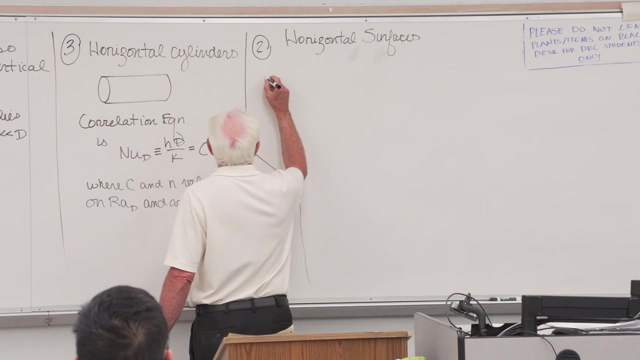 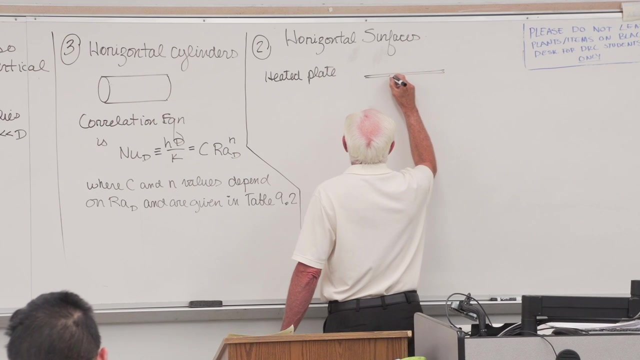 Now we take the harder, We take the harder one: Horizontal surfaces. So with our horizontal surfaces we can have first of all plate, If the plate is hot and the fluid is cold. let's just use air as an example. 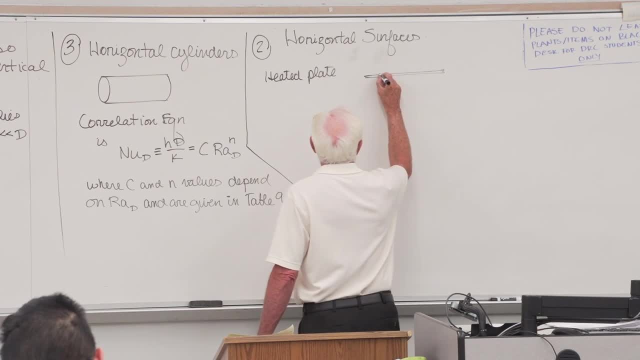 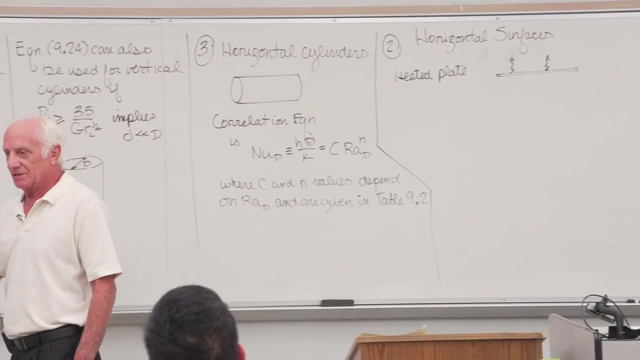 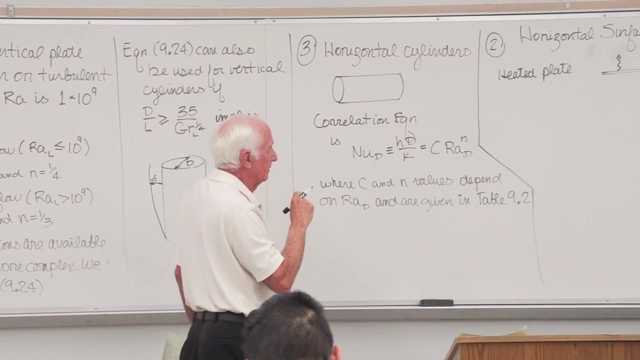 If the plate is hot and the air is cooler- and I mentioned that, the asphalt street- in the middle of the day, when the sun's being down on it, you'll see, though, the wavy air patterns off the asphalt street. Same thing here. 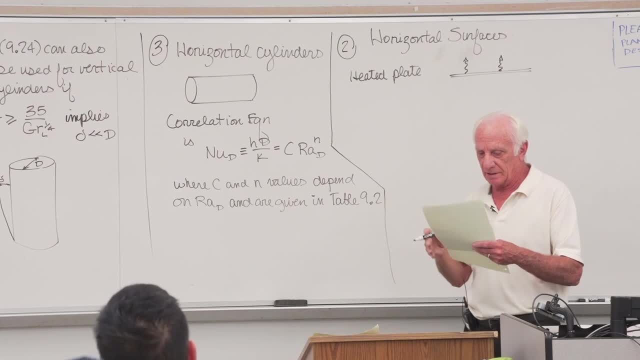 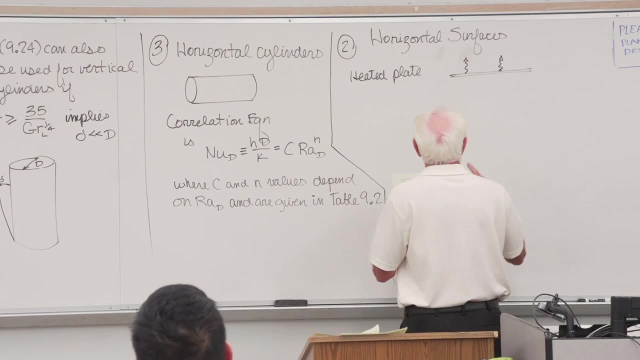 That's free convection heat transfer. if the wind's still calm days On the bottom, there can also be some air. down there It's being heated. The air is getting hotter. It's getting hotter on the lower part of the plate. 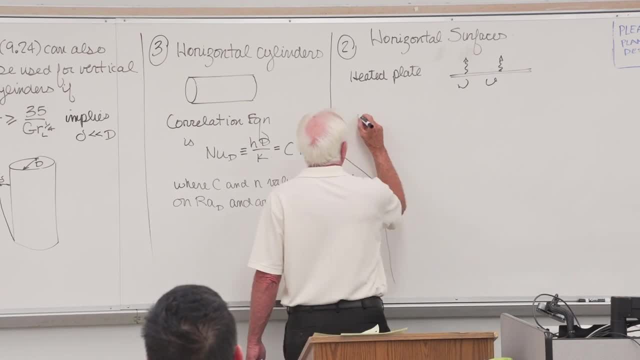 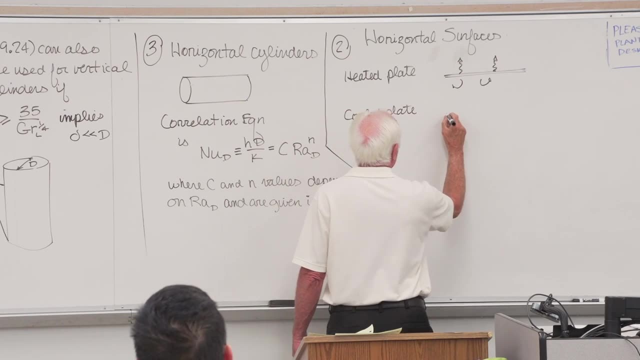 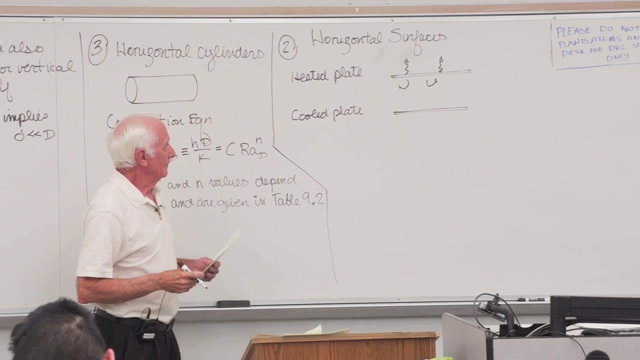 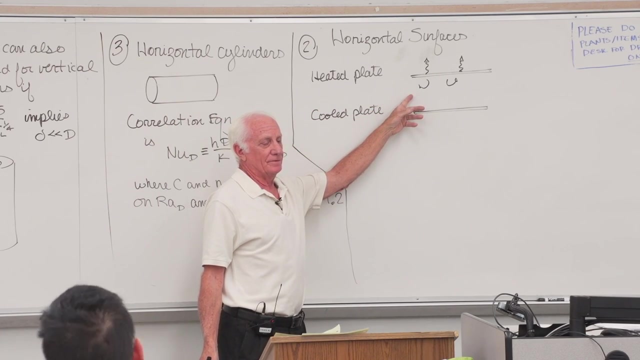 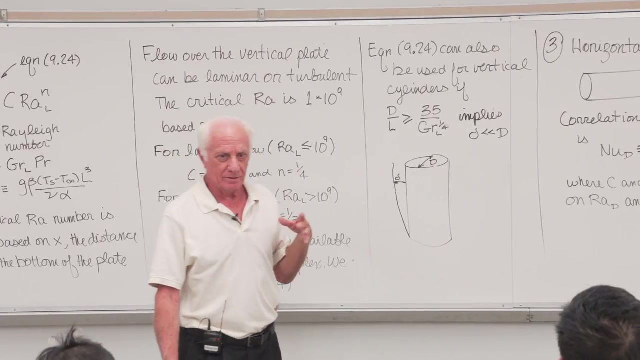 And then we have a cool plate, By the way, on the top one up here. you know where the best heat transfer occurs: on the top surface. On the bottom it's like you've got an insulating layer, So the bottom is not a good. 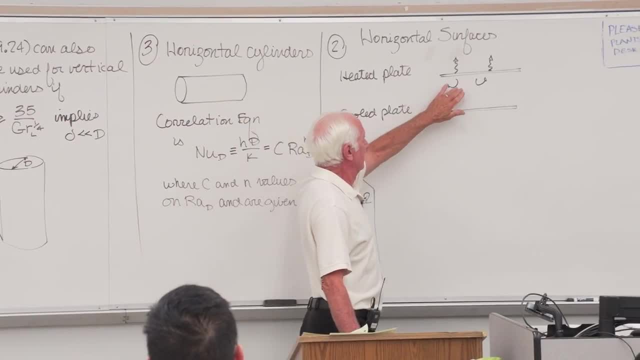 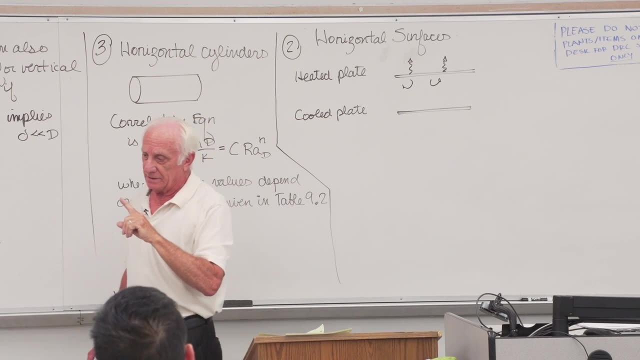 you're not getting good heat transfer because the air close to the plate has been heated and it can't go up. It wants to go up. Its density goes down. it wants to go up The buoyancy effect, It can't go up. 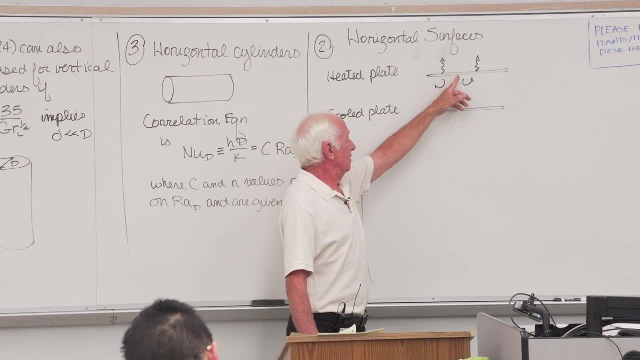 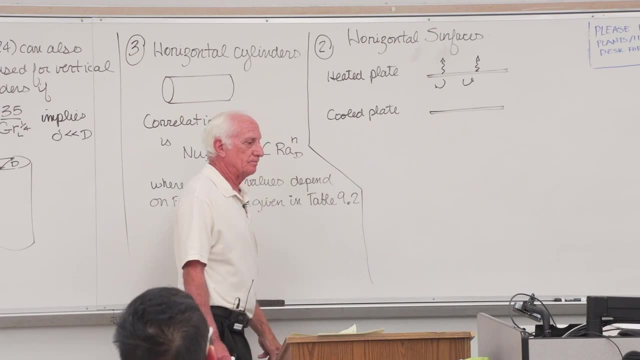 There's a wall here. The top is just the opposite. The air close to the plate gets heated. Its density goes down. it wants to go up? Oh, it can go up. Good heat transfer. Now the cool plate, The cool plate. 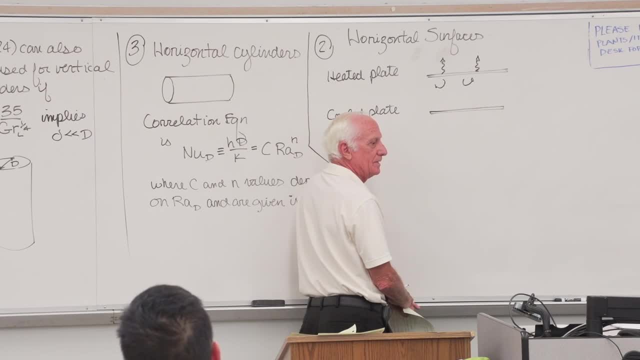 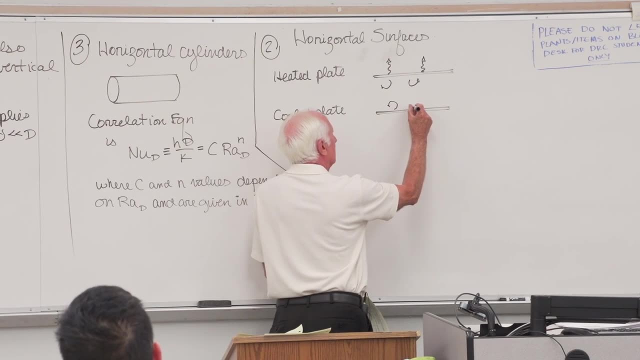 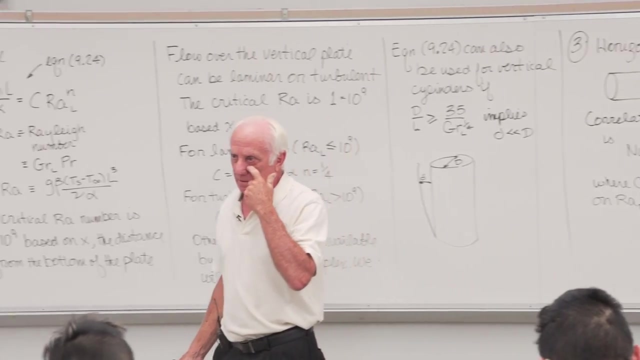 Air molecules on top get cold. Density goes up, More dense. air wants to drop. It can't drop. There's a wall here At the bottom. the air molecules touch the cold plate. The density goes up. They get more dense. 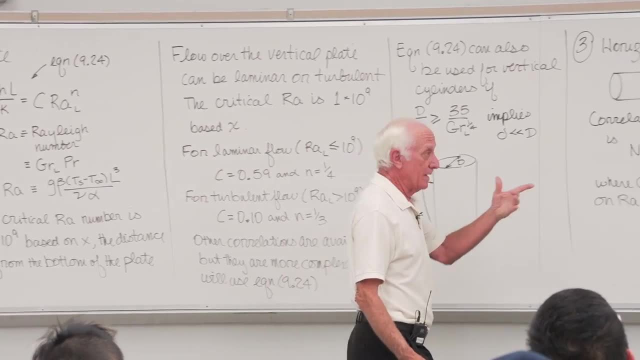 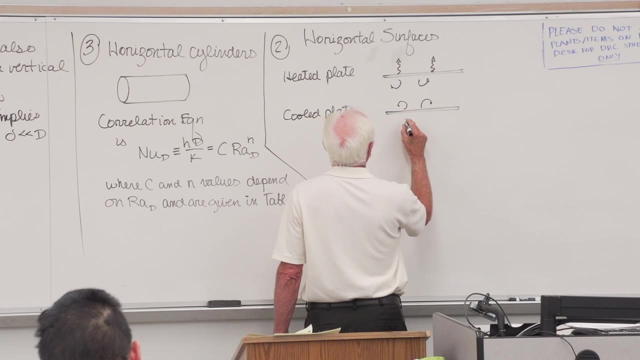 They want to drop because they're heavier. Oh wait, they can drop now. They can drop now. So cool plate. So yeah, in this case we've got the cool plate. So yeah, we can just go ahead and show that. 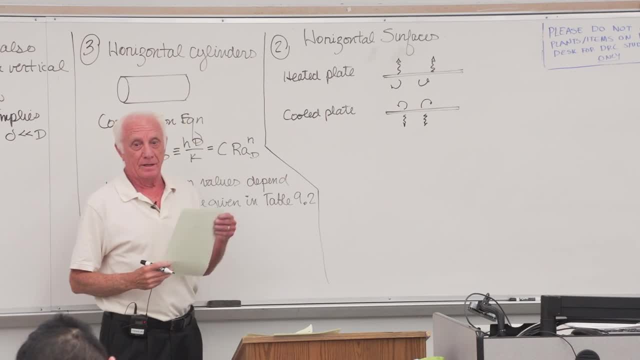 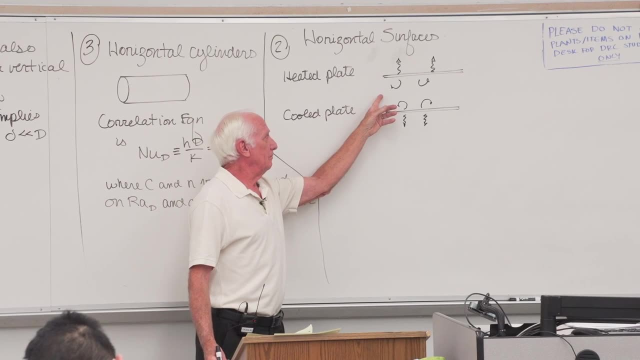 Well, why is two more complex? There's four possible H's: Heated plate top. find the H. Heated plate bottom. find the H. Cold plate Top. find the H Bottom. find the H. Four choices. 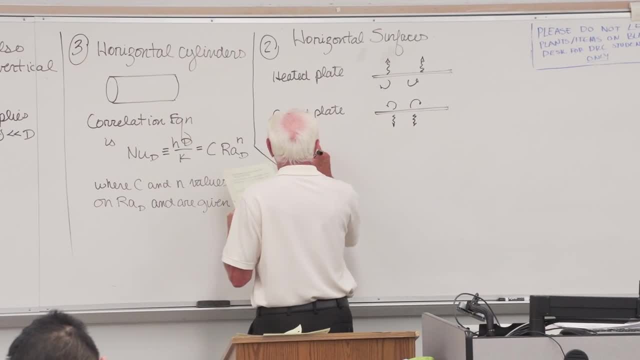 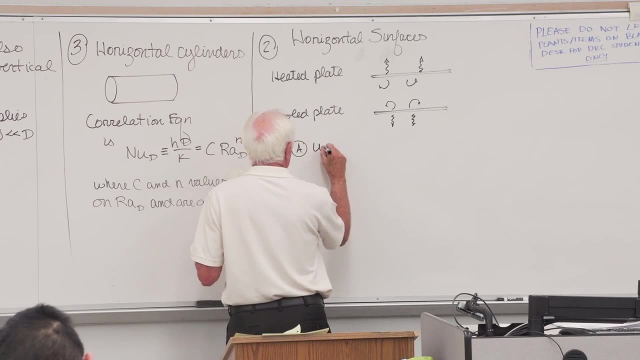 So let's take them one at a time. So we'll do, let's do- I don't know. we'll do A and B. A upper surface of hot plate. A upper surface of hot plate. A upper surface of hot plate. 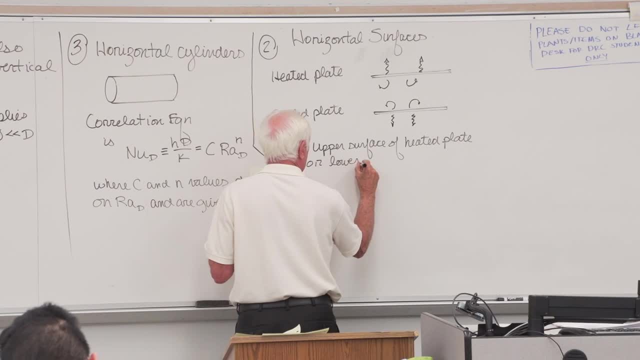 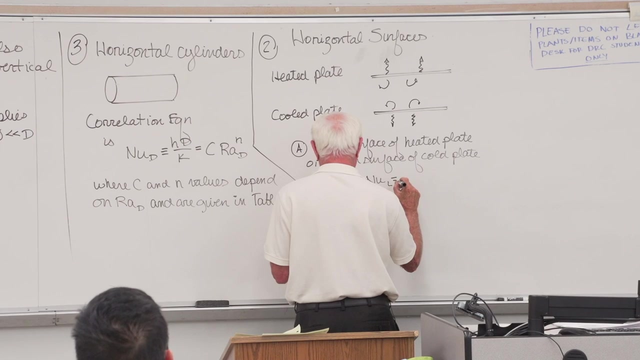 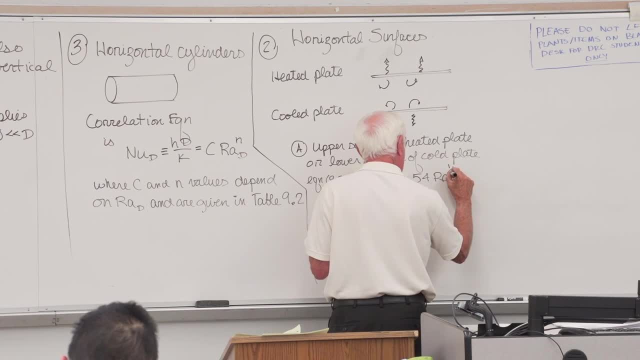 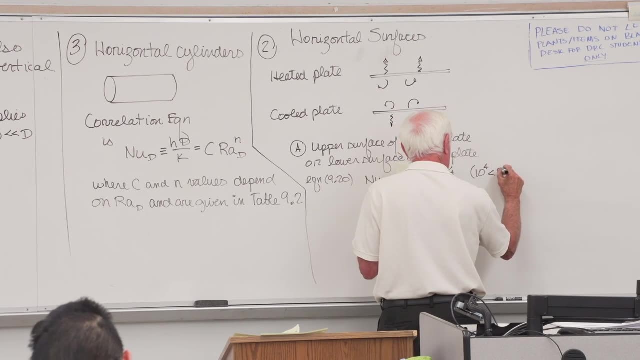 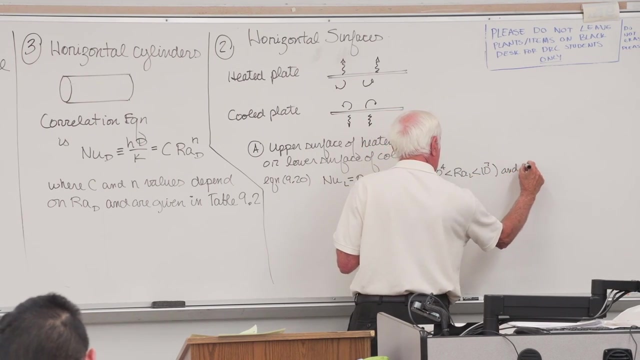 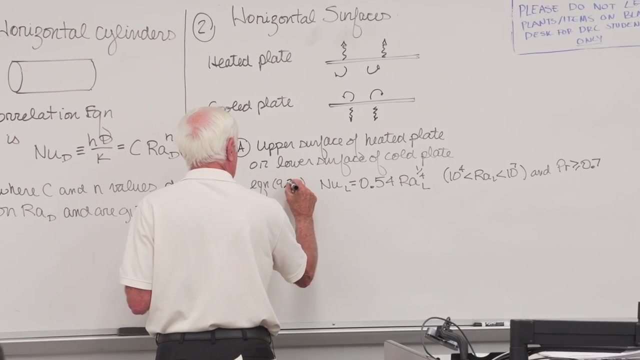 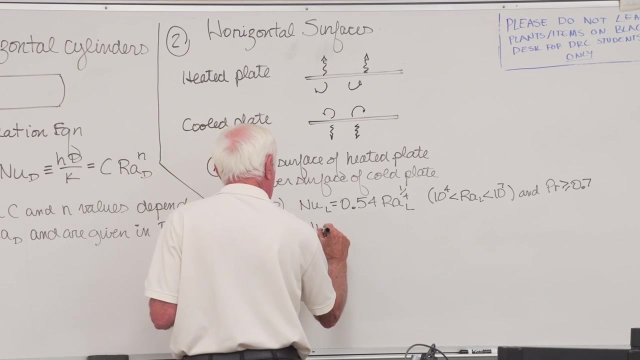 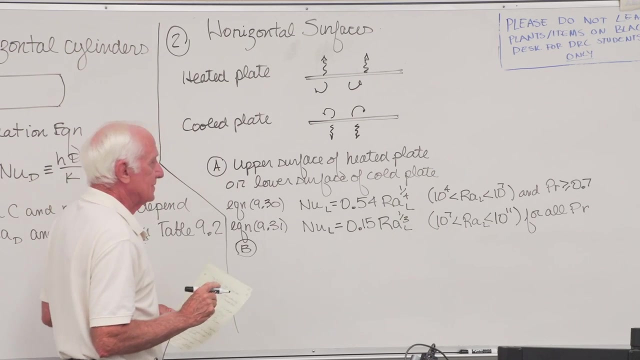 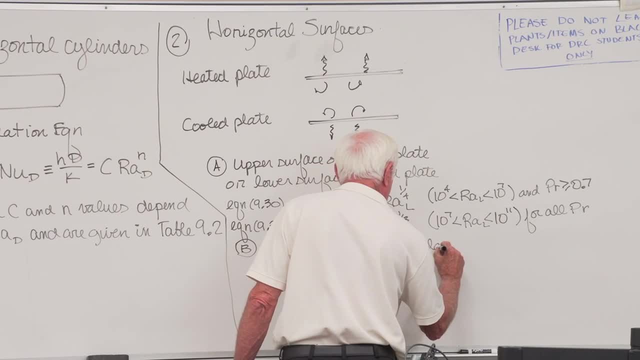 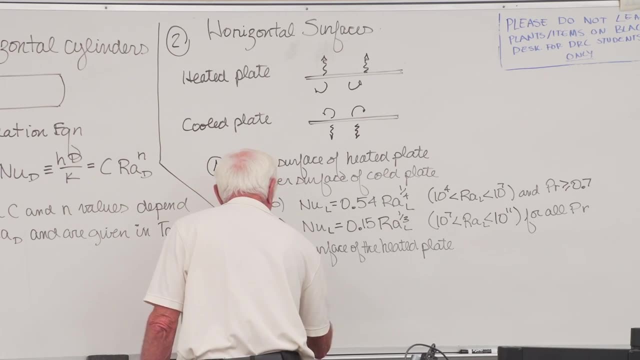 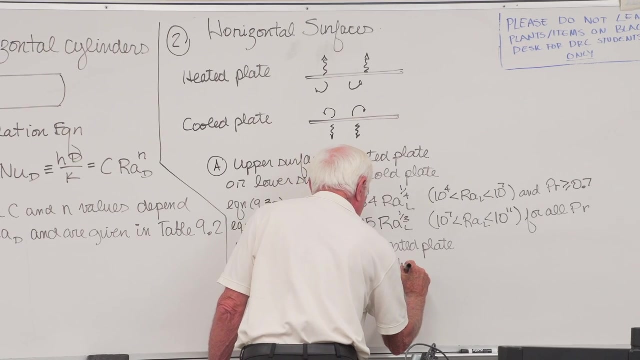 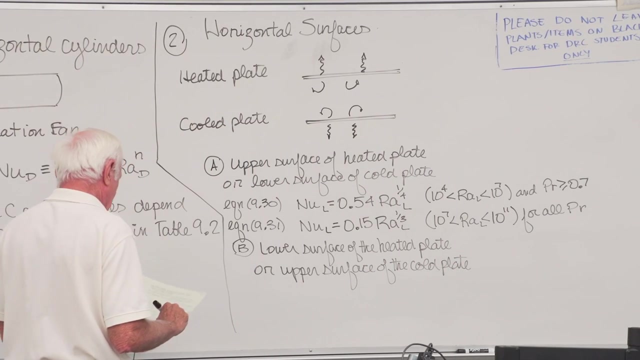 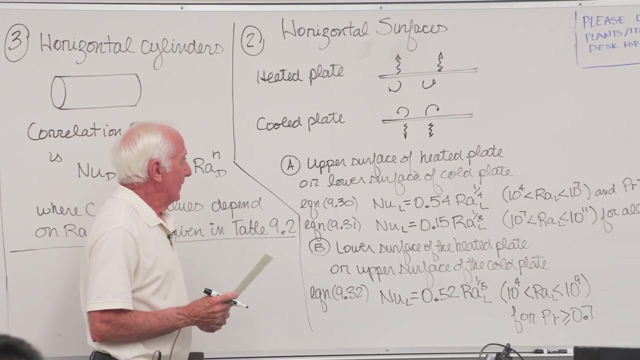 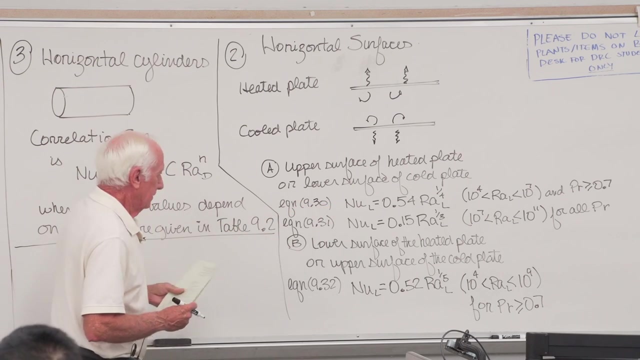 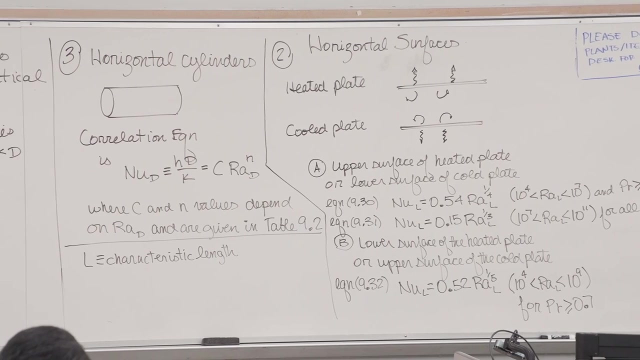 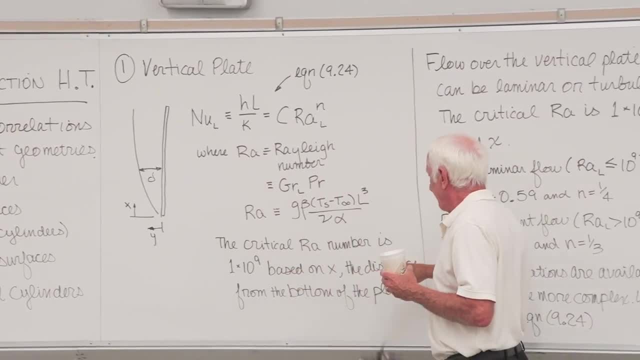 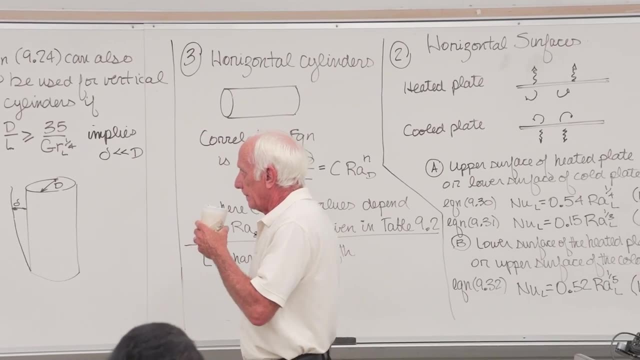 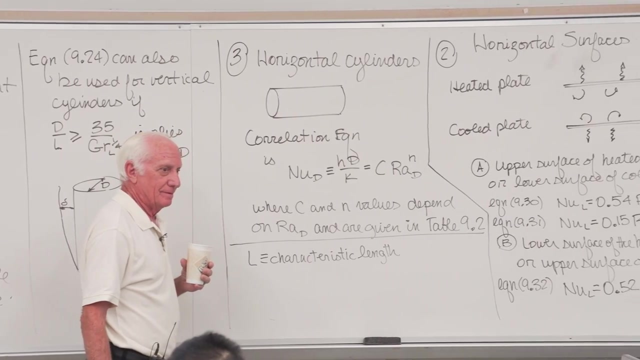 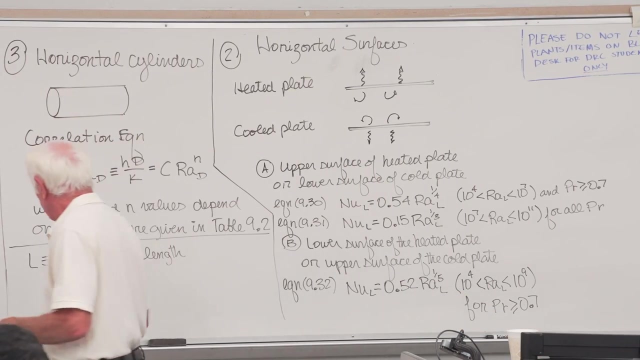 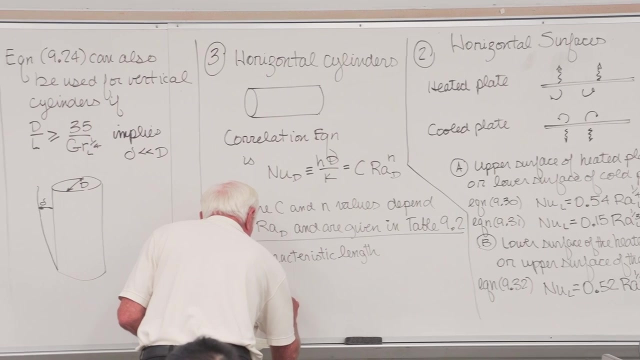 Vertical plate L is top to bottom. Vertical cylinder L is top to bottom. Now we have something called the characteristic length. So our characteristic length, L is defined like this: L, L High, and keep Mo misses L, L Velvety or L high. 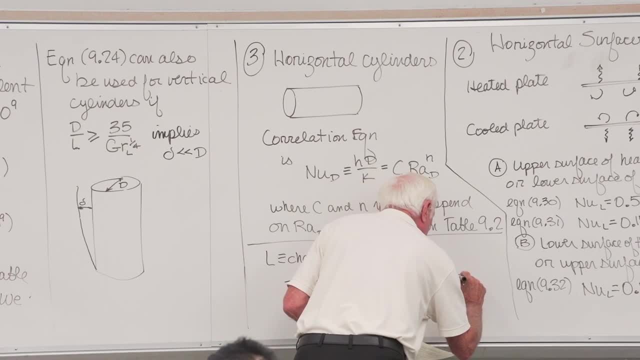 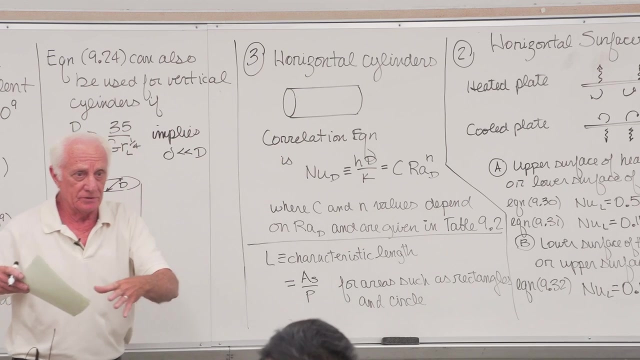 L, 12, L and L, Mid lF and lL, V, L, lV, mR, M. Let's try L. Let's try this one again, where our constant, our faster composer gets to M. 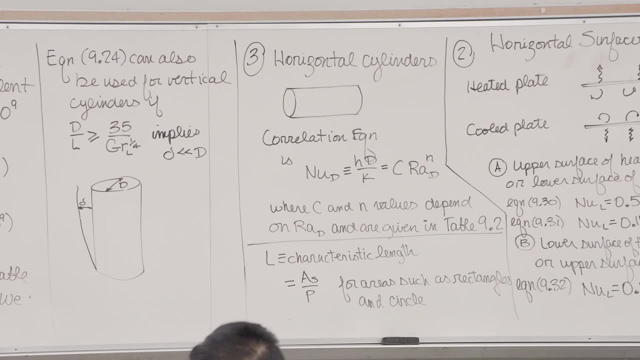 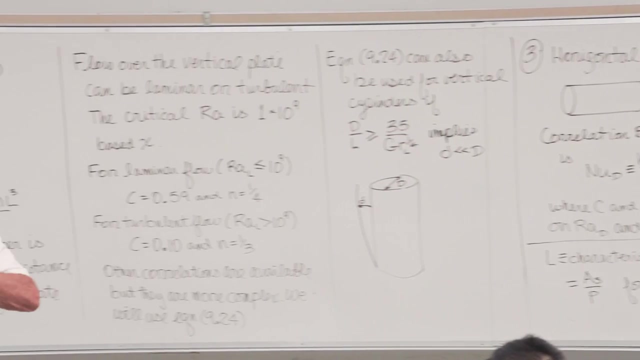 So if we B and L, m to find L, to put L in the Nusselt number and the Rayleigh number. this is how you do it. You take the surface area divided by the perimeter. If it's a circular area, surface area pi D squared divided by 4. Perimeter: pi times D. 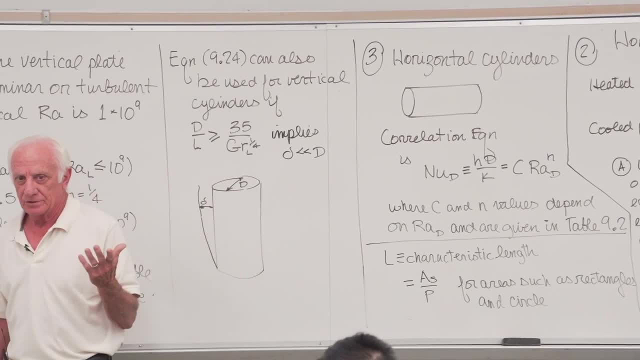 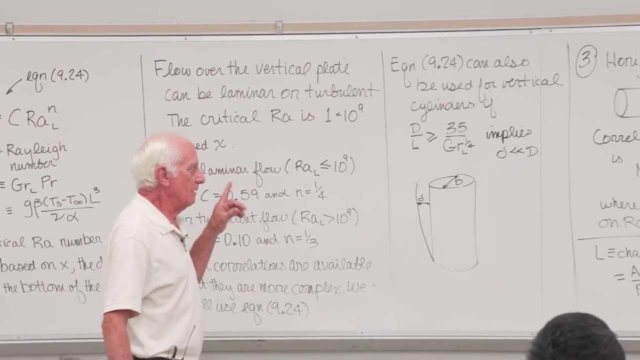 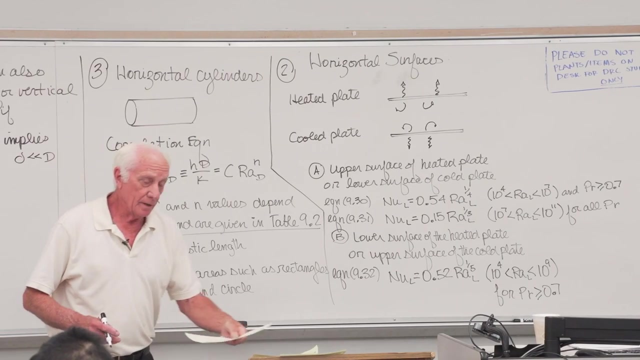 divide them out. You get D over 4 for a circular area. But for each area that you've got, find that characteristic length, L, Then put the L in the Nusselt number and the Rayleigh number and solve for H. Yeah, you've got to make several decisions. Now life is a lot easier. 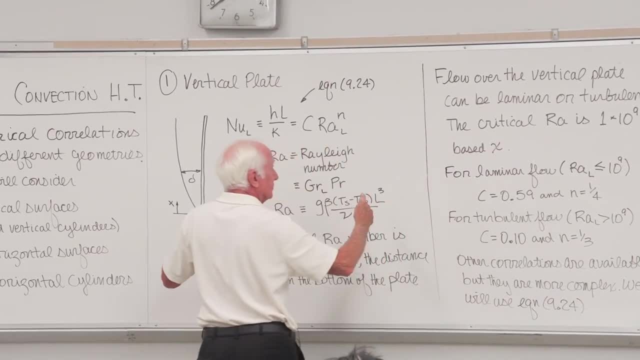 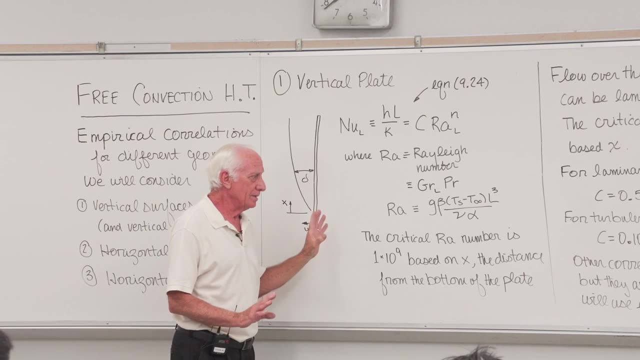 for these vertical plates and vertical cylinders, because there's one equation I'm not going to go wrong in this class. There's more complex ones, but we're not going to try and look at the more complex ones. We take the Nusselt number and the Rayleigh number and solve for H. 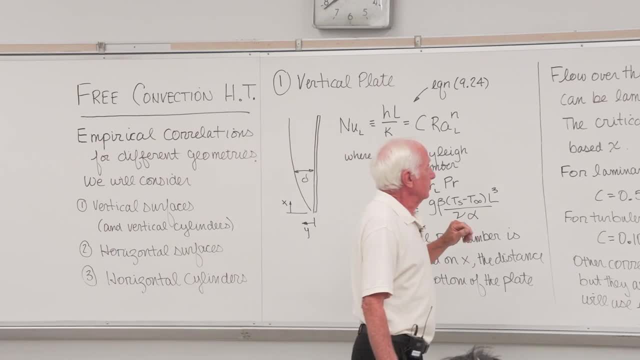 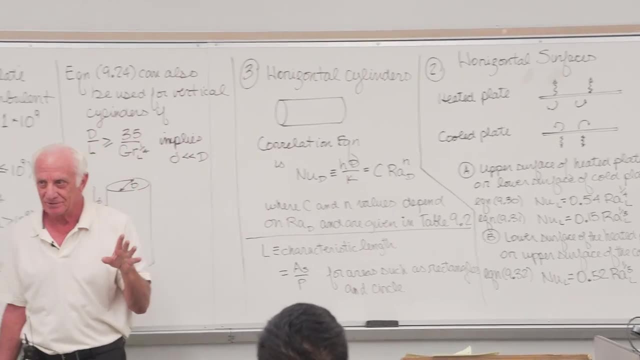 So you can find that characteristic length L. Then put the L in the Nusselt number and the Rayleigh number and solve for H. Take this one and use this one, Okay, horizontal cylinders. You've got one choice There. it is Not a problem, Use that one. 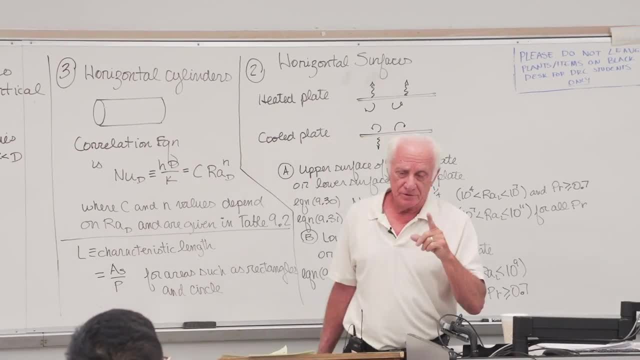 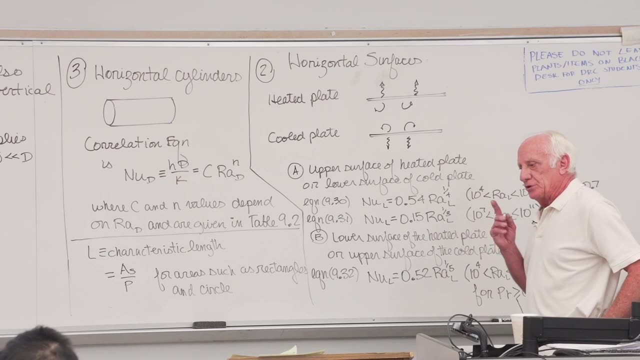 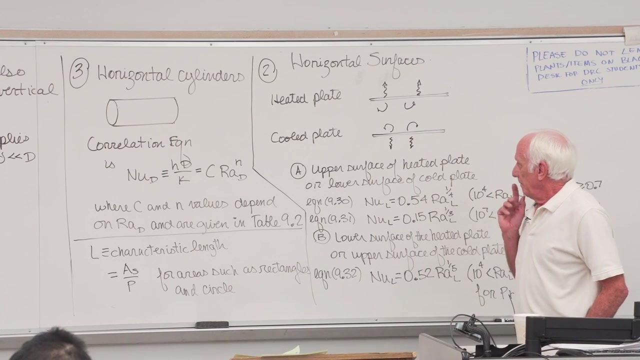 Now you've got a horizontal surface. The first question: is the plate being heated or cooled? Okay, answer that first. Number two: are you looking at the top or the bottom of the plate? Got it? Number three: check the Rayleigh number In this range, that equation In this range. 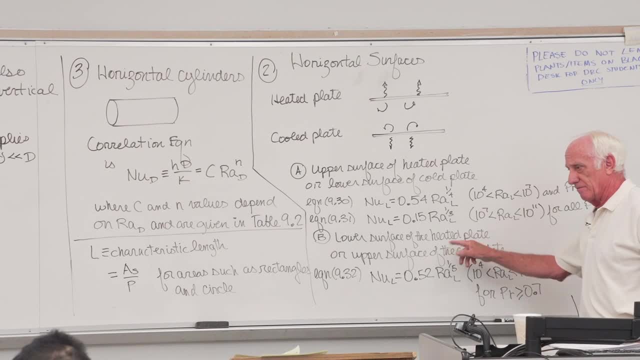 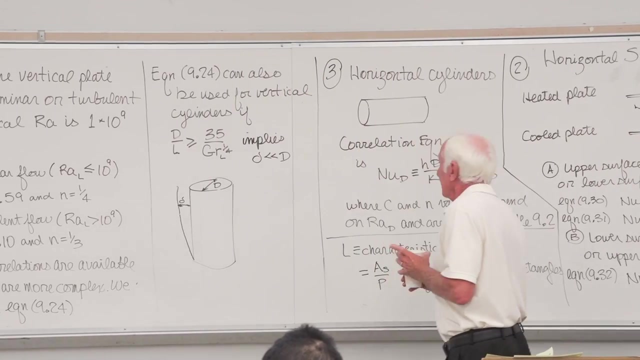 that equation For B doesn't matter, One equation for both, So you've got to really make three decisions. on number two, horizontal surfaces. Okay, I think we've got that All right. any questions on these guys then? Okay, 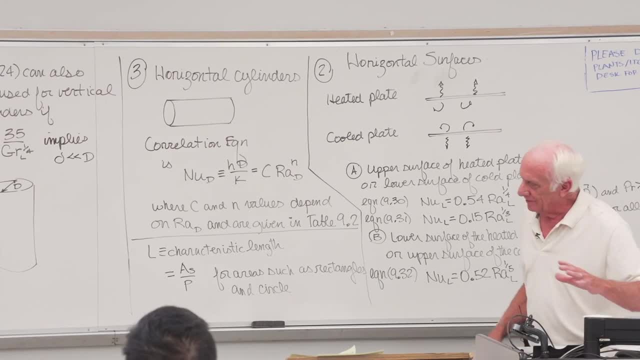 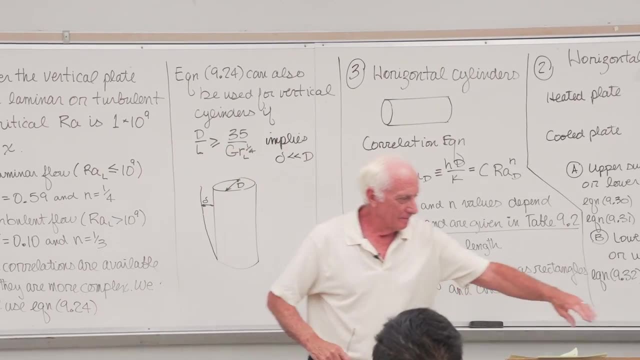 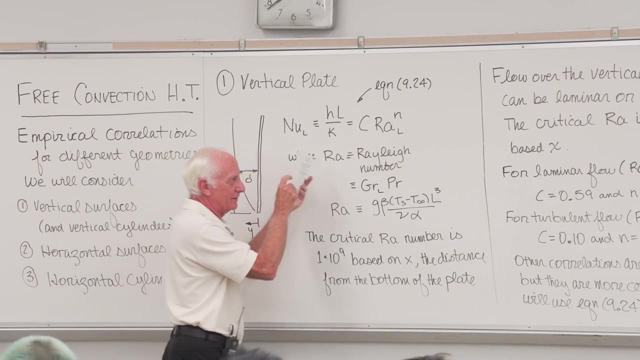 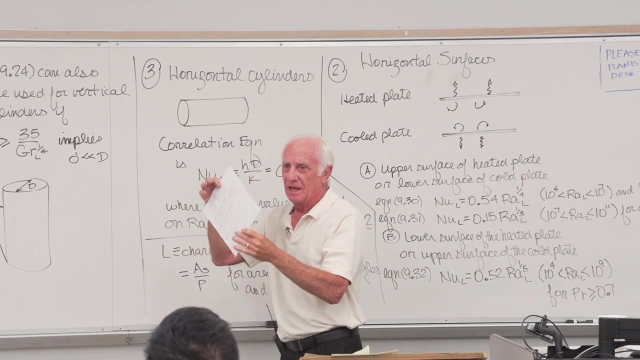 I mean, you have to get at least three different questions. So well, there are other geometries too. Here's a vertical surface, Here's a horizontal surface. You want to be more complex? How about a 45-degree angle?